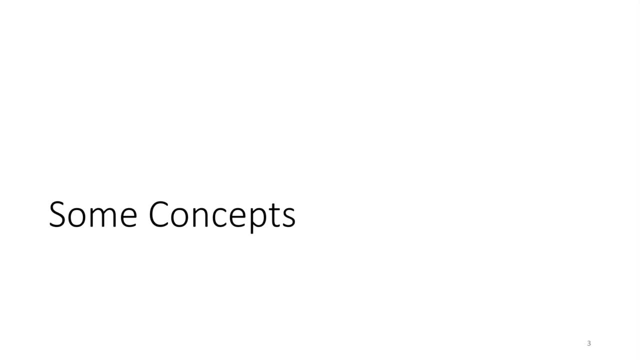 like to give that to you so that we can understand what kind of application we can use this concept. Okay, so the first thing is that I will start with, even right here, a person and then this person, because always when we do the control, actually we can do the manual control, human control, 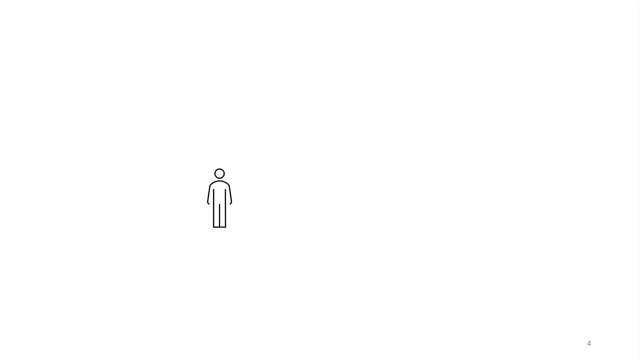 for example, we can do anything We can do. driving, we can do whatever. yeah, but how can we turn this into machine learning and with it, Okay, now just a simple example that every day we are going to do, for example, big. 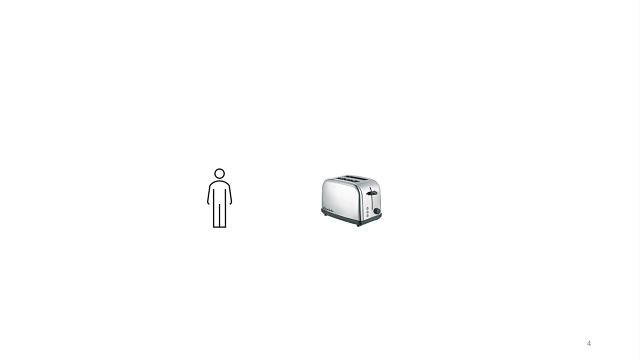 toast and then so we put two pieces of bread into that. How do we control? How do we make sure that the toast is good enough? And then? so, if we do not have any feedback, for example, one thing we can do is that, actually, you can point the timer in the machine learning mode. So, if we do not have any feedback, for example, one thing we can do is that actually, you can point the timer in the machine learning mode. 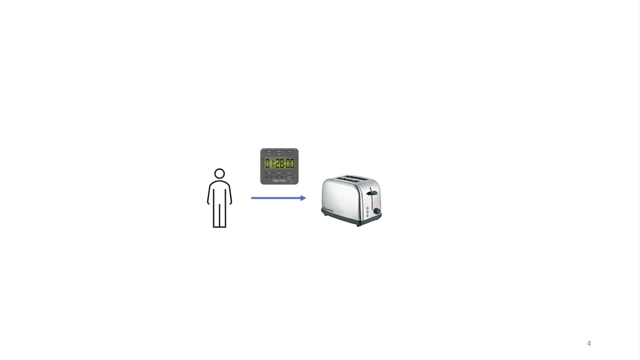 So if we do not have any feedback, for example, one thing we can do is that actually, you can point the timer in the machine learning mode. So what we are going to do is that I just set a timer, for example, one minute. 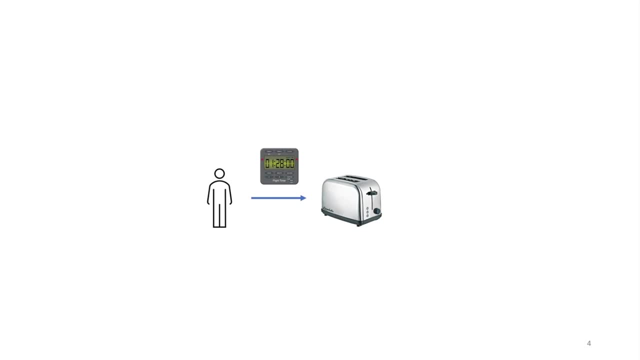 20 seconds and then so stop, and then I'm going to look at the toast to see whether it is good enough or not. So this kind of thing we call this is the open loop system. We are doing the open loop control, but the thing is that again we do not know whether it is good or not, So we are going. 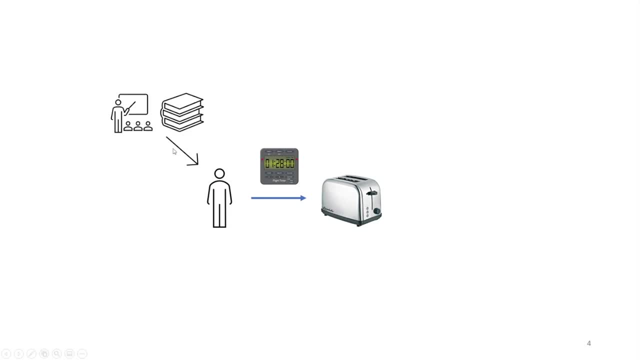 to do some learning. This kind of learning is that so we can do some experiment. We are going to do some experiment, We are going to try this many times and then finally I'm able to get the timer right here for the right time and then. so this is a kind of human. 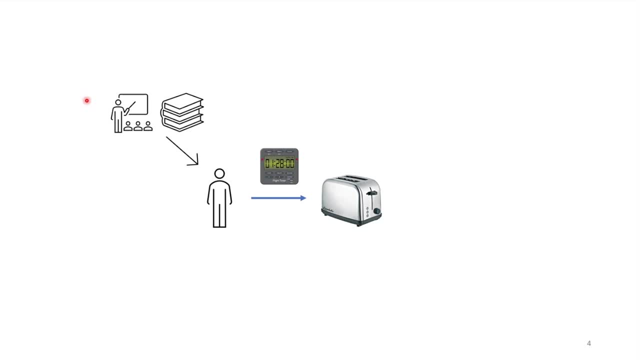 learning, and then this is very similar to machine learning, But the thing is that this is the open loop system, and then so it is good that after we learn all these intelligence, or learn all these groups, it applies in the earth, But in we are going to move to another enrollment, for example class, because we have to learn. 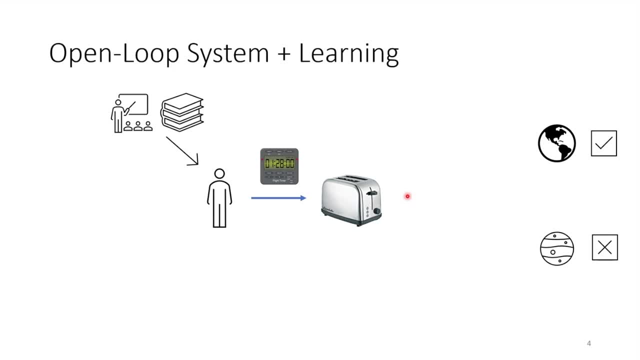 everything again. So this is open loop system and learning. and then now I'm going to talk about another concept that would be just the same person at the same time. Maybe this is me and I'm going to do the same thing Now, this time I'm going to use my nose, my eyes to look at those. 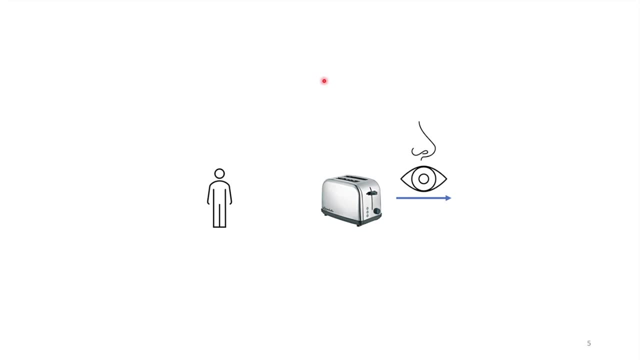 toasts to see whether the smell is good enough or the burning condition is good enough or not. So I'm going to fit this back to myself because I look at that, I smell that, and then I just know that whether it is good enough or not. 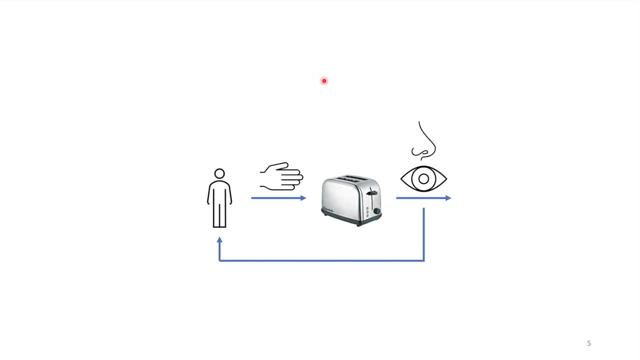 So if the smell is good enough, I'm just going to press the stop button and then this is the closed loop system. So we will just have look at the condition and then go back to myself and then I'm going to determine whether I'm going to stop the toaster or not. Okay, so this is. 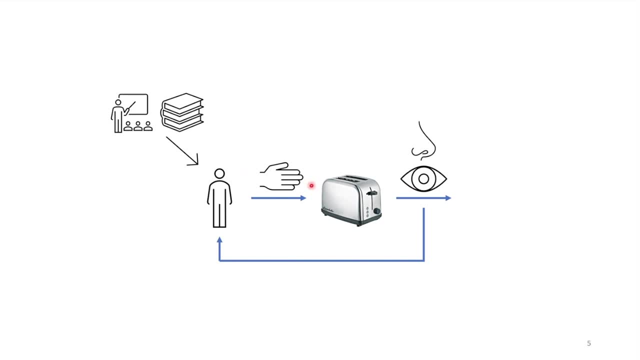 so how do I know that, when to stop? There are two ways to do it. I'm going to have to buy more knowledge so that I know when to stop, because I know what kind of smell it indicates it is a good toast, or what kind of color it indicates it is a good toast. If it is not, I'm going to have a. 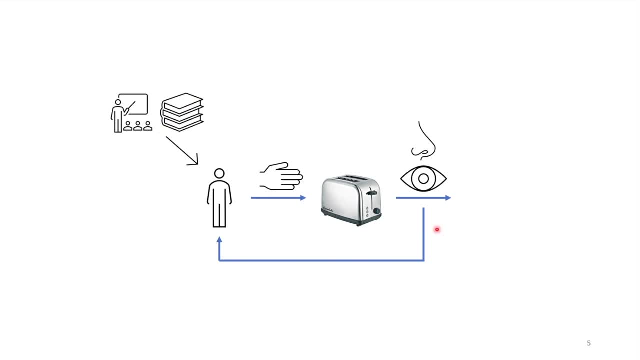 learning outcome. This learning outcome that is, through this I'm going to have, say, a route to tell me that I'm going to do this routine and then I'm going to give that to expertise, and then they tell us, they tell me that whether this is a good toast or not, and then, through that process, I'm going to 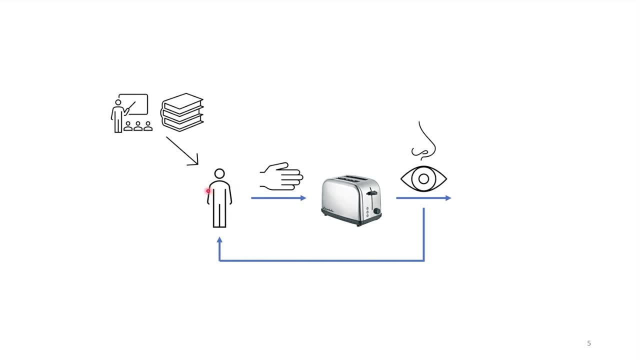 learn that, and so I will have to control policy to tell you when to stop the toaster. So because we have the feedback, because we have the sensors right here, so most likely it will be more robust. That means in in different enrollment it is possible to have more or less the same result. Okay, so this is. 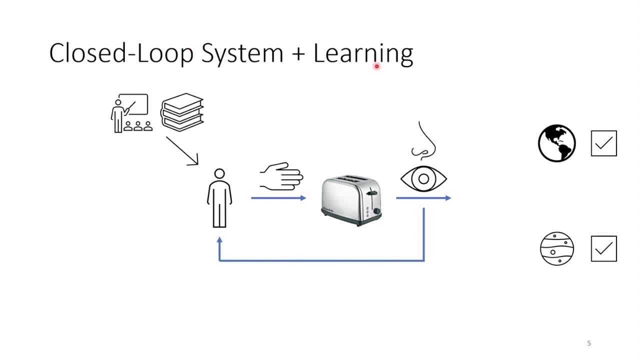 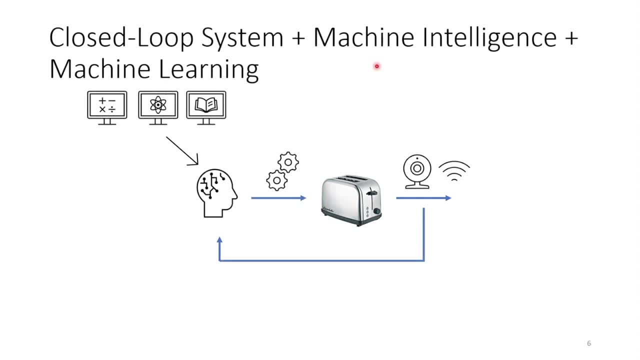 something about the code loop system and learning, and so we combine them together. but up to now it is still about the human learning We just learned by ourselves. but how can we turn this into machine intelligence? and then? so we exactly use the same framework. The only difference is that so 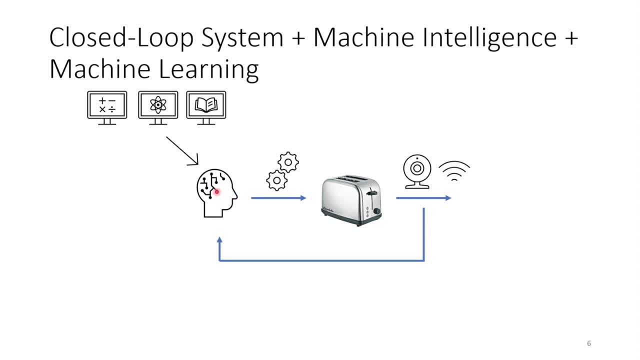 we're going to replace the human by using a machine. This machine could be a computer, it could be an algorithm. So we have something right here to implement the rules or the policy when to stop the toaster, We still need to have something that would be some actuator. actuator that means that would be some mechanism. 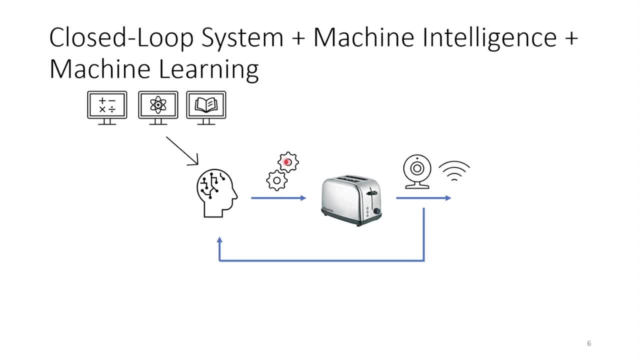 to stop the cold toaster. Maybe we have a whole water finger to stop something like that. and then at the output we have the sensors. These sensors that could be a red camera or some whatever sensors We are going to sense the right information that will be fed back to. 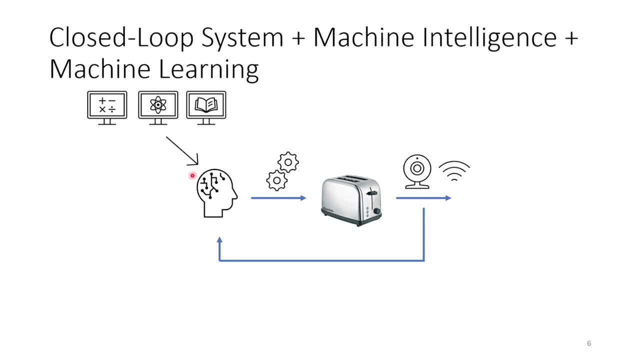 the machine to make decision. So we call this the code loop system- machine intelligence. and then on top of that we have some learning algorithm which is going to learn this intelligence, so that we develop intelligence to tell when to stop. Yeah, so this is the main. 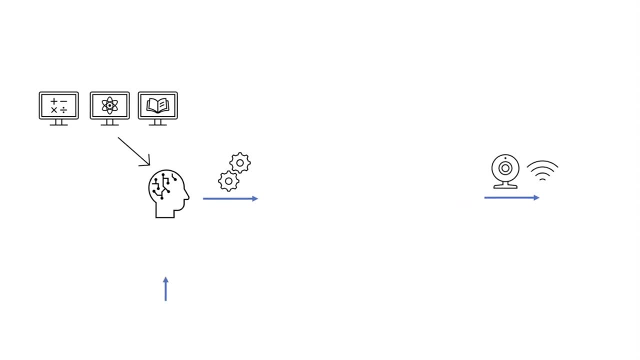 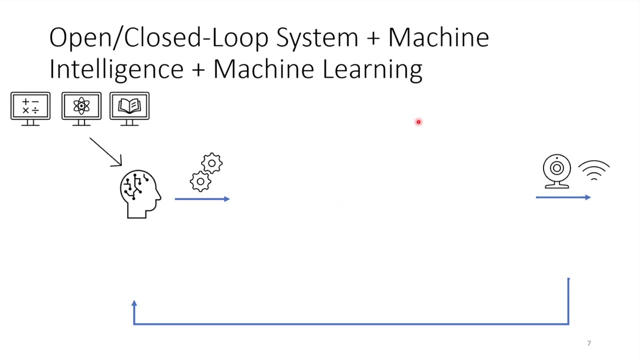 root of the code loop system. Now i'm going to expand this, to expand it a little bit more, and then what kind of applications we can use this framework. So I've just used the icon to represent that Before I'm going to present some videos to you to demonstrate what kind of 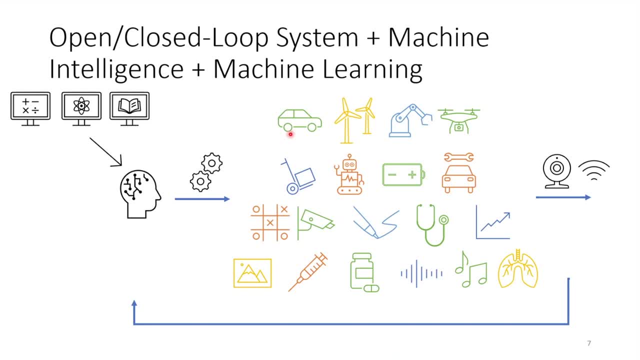 we can have. For example, we talk about self-driving, the driverless, autopilot driving vehicle. So the same thing is that we use the sensor, This sensor which is able to capture the location, the velocity, whatever thing, the obstacle in front of us, And then so we know this. 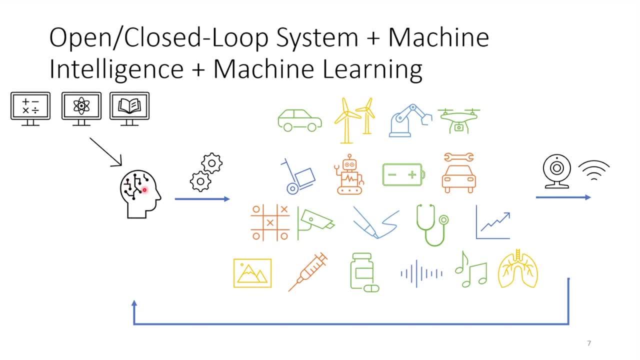 information, Put it back into the machine. The machine may be located in the vehicle or somewhere else, And then so this signal, the control signal, will be transmitted to the vehicle to tell the steering angle, the velocity, so and so, whether there will be. 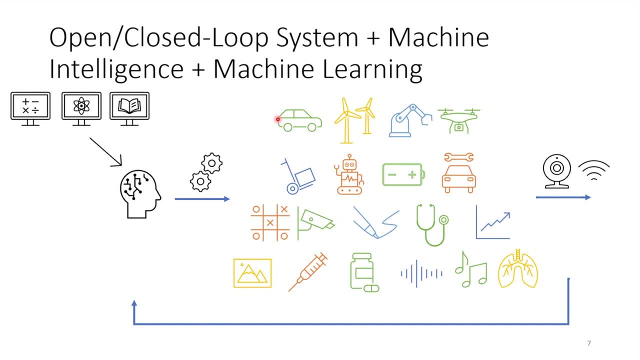 some obstacle in front of us And then we are going to stop or not. And then so you can see that this is the cold-sleep system. And so another example: there will be some wind turbine system, And then so we can use exactly the same framework, That is the cold-sleep. 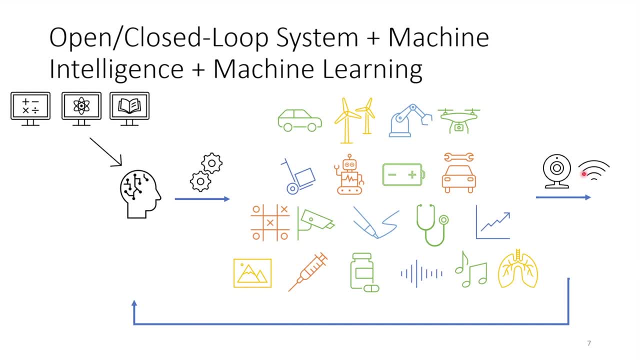 system right here. So we are going to control the power generated. The power generation, it depends on the wind. The wind is very strong And then we do not want to damage the wind turbine system. We are going to turn the weight into different angles so that the speed of the wind turbine 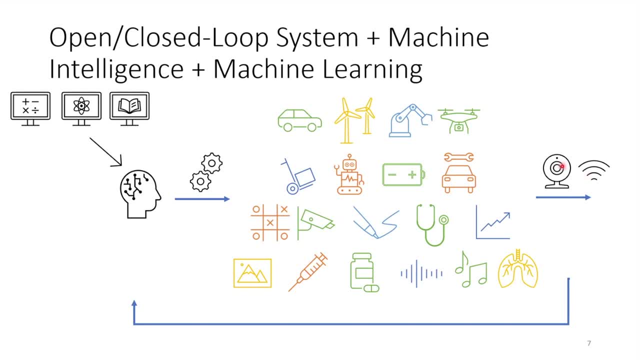 can be controlled according to the sensor's information. And then we get back to the controller in order to determine what kind of wind turbine we are going to use, What kind of angle of the wind we are going to adjust, so and so, And then so on top. 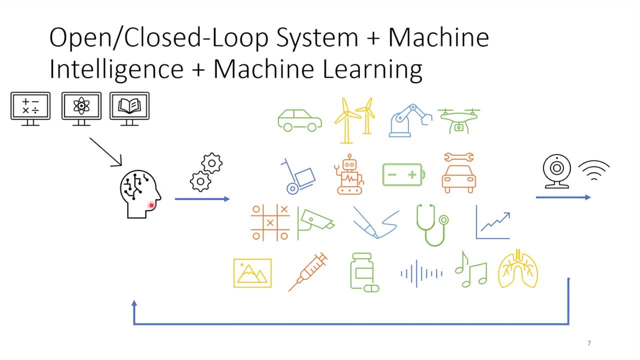 of that. so this machine- intelligence- or this machine actually it is not- even can do the control. It cannot do a lot of things, For example, fault detection. That means when we are going to want the wind turbine system, when the wind turbine is turning. 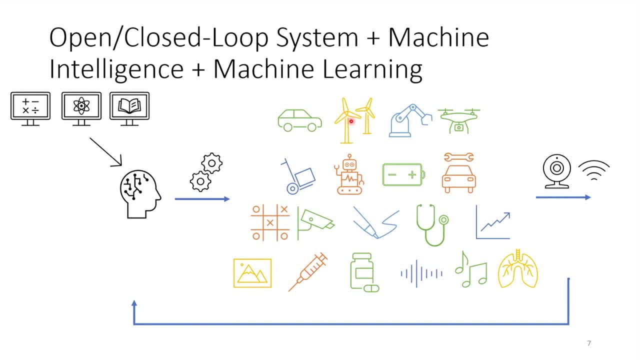 and then so we can call out this signal, This signal, we can look at this waveform and then so we are going to determine: look at this waveform, and then we determine what we are going to do for the wind turbine, whether there will be some something wrong happened. 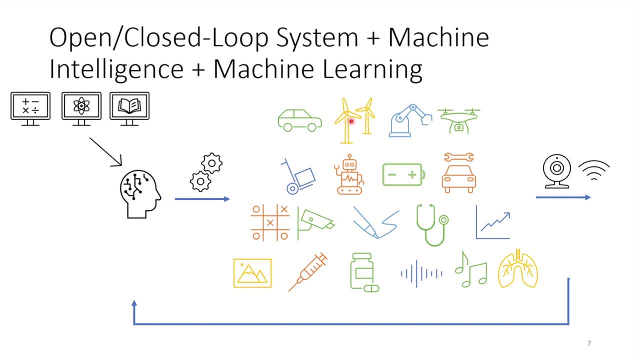 If there will be something wrong happened, we are going to send this signal to say the rescue team or the wind turbine's team to fix the wind turbine before it is fully damaged or it cannot be. it cannot function. So we have a lot of things, For example, 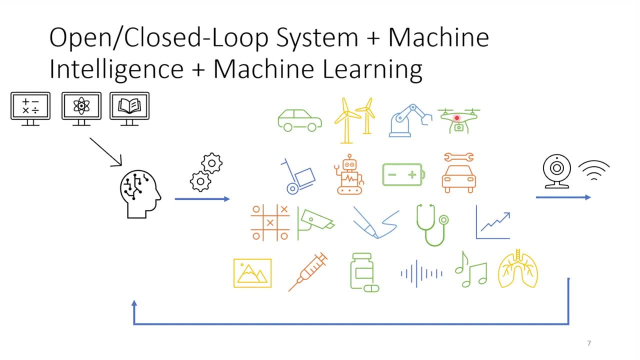 the robotic arm control control for delivery in the warehouse system and then so for whatever power system, say, we have the electric vehicle and then so we have a patch of battery. We would like to manage the power consumption because all the battery, the battery. 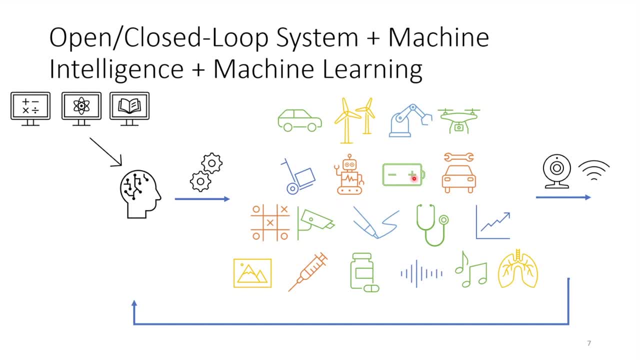 pack has a lot of battery inside, and then they have to work together, Otherwise they will overheat. So we have to have many management systems to make sure that the battery work together in order to produce The required power consumption. I mean the power generated. we can use the machine learning. 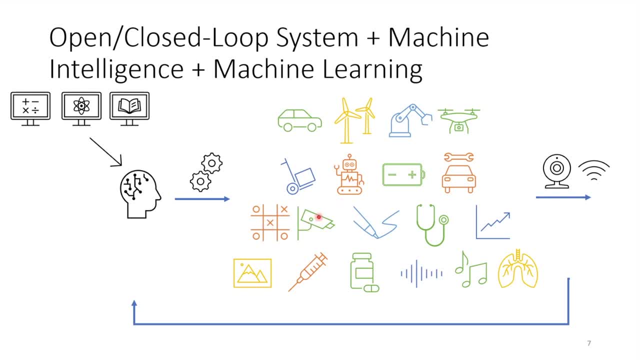 to take in, and then so surveillance system, and then look at the gate or the poster of a human to determine whether this activity is whatever. to recognize the activity, yeah. And so say job administration or job discovery, yeah. so we can do something like use the 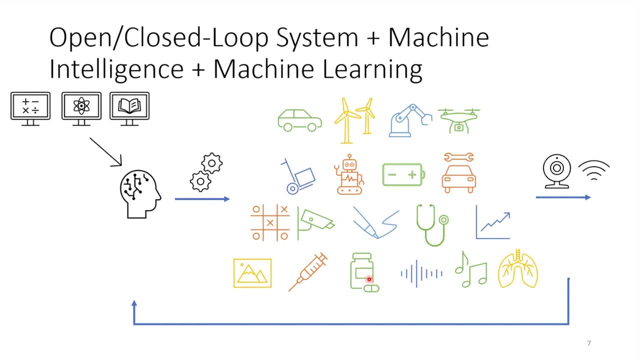 chemical, to represent that as a graph and then so feed it into, say, machine learning algorithm to determine whether this, whether this drug is, I mean, can produce positive effect or negative. yeah, So that is something, yeah, we can use the machine learning to do. 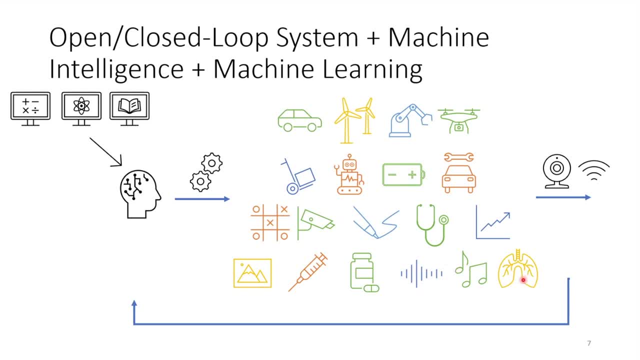 that, And so music composition or even something like the COVID lighting detection- I'm going to talk about that later. That means with this framework we can do a lot of things. the COSM system plus the machine intelligence, plus the learning algorithm, right here. So I'm going to summarize a little. 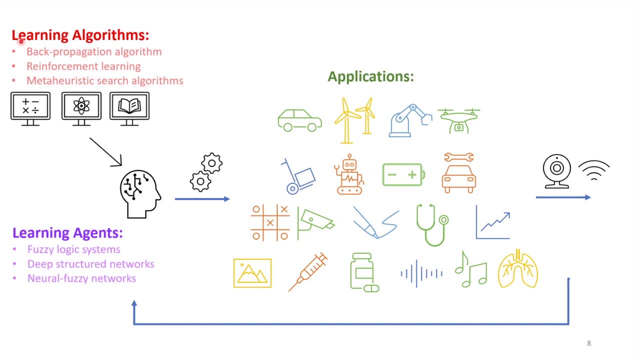 bit what I have just mentioned. The first thing is that we have some learning algorithm right here to tell the machine how to learn and then so we can have a lot of algorithms just laying a few, say, back-publication algorithms. 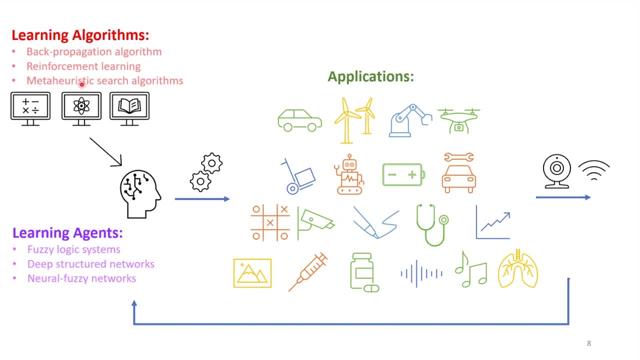 We can have some back-publication algorithm, reinforcement learning, or some metaheuristic search algorithm, for example genetic algorithm or particle swarm optimization. yeah, And so that would be learning agent. this learning agent that is, you can regard it. 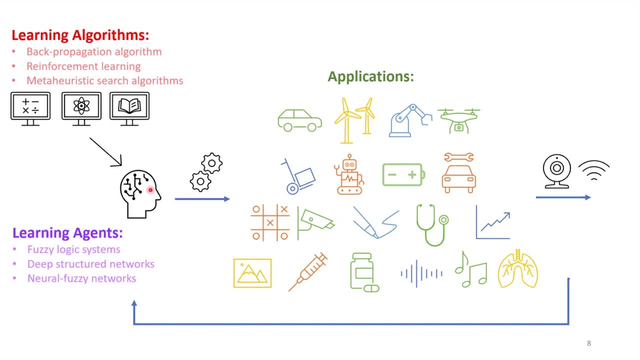 as a mathematical function, but some mathematical function will have better expression capability, So we demonstrate better learning capability. For example, we can use first logic system or deep structure network or so and so So in the middle we will have the applications. 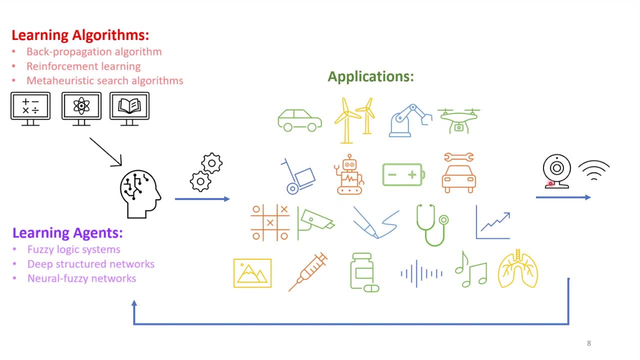 In between, we have the actuators as well as the sensors, and that we're going to close the feedback loop or we can open the feedback loop. It depends on what kind of application we're going to do. yeah, So now what I'm going to do is that just to explore a little. 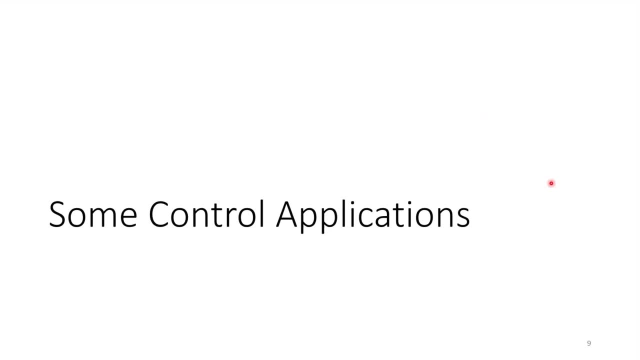 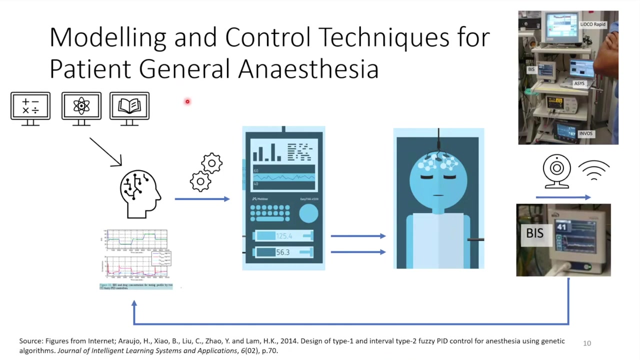 bit about some control applications So you will know what we can do using this kind of framework or mechanism. This is something my team has done, that is, using some machine learning for modeling as well as control for the patient in general. We have done that in the Keynes Medical School. 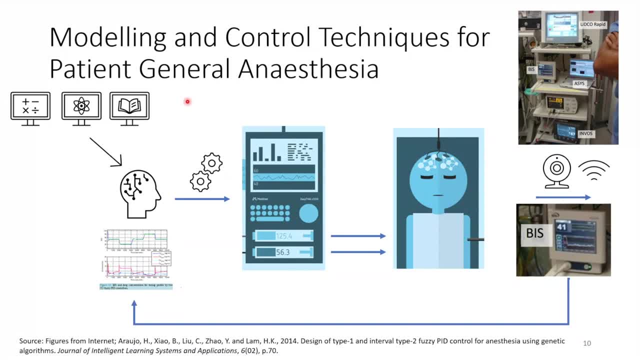 many years ago. I cannot remember how many years ago, But anyway, the idea is that we have a patient right here. We would like to inject drugs into this patient in order to put this patient into sleep, So we have some setup right here. 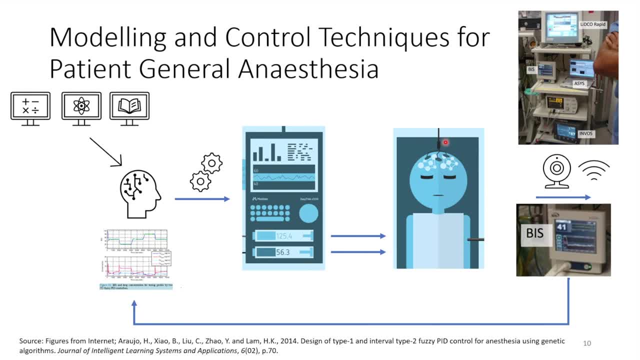 We haven't done the clinical trial, but this one, that is, we have a simulator there and then compare with the real patient and the response of the real patient to see whether he works or not. yeah, In this figure we have the treatments right here. They're going to collect the data. 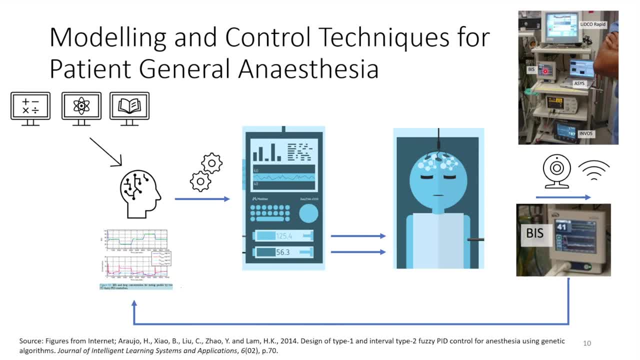 as well as the most important thing that is about this piece, that is, the bisexual index, which is an index to measure how deep the patient is sleeping. okay, So we would like to construct the index in the value about 50.. So this is the general and the 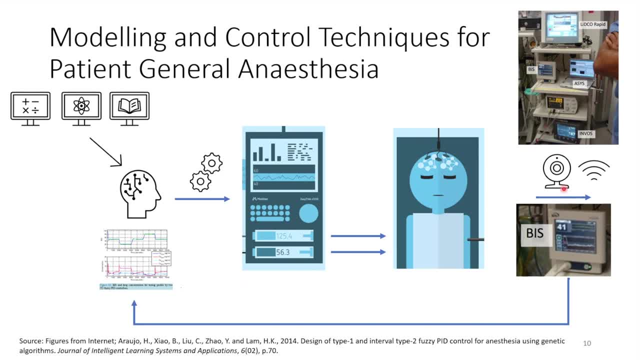 settings are going to make it a little bit easier. We would like to. actually, the idea is that we are going to have the learning algorithm to learn to control policy. This learning control policy will tell us what kind, what concentration of the drug will. 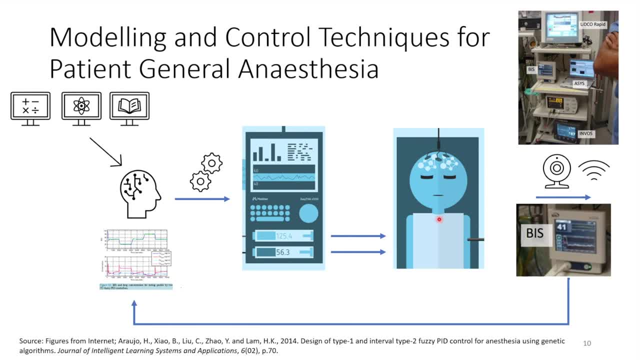 be injected into the patient. We are going to control concentration of 2 drugs, The first one that is foliprofacor, and the other one that is the when we fatal mel and then. so So we can just simply inject that into this patient and then we can put. 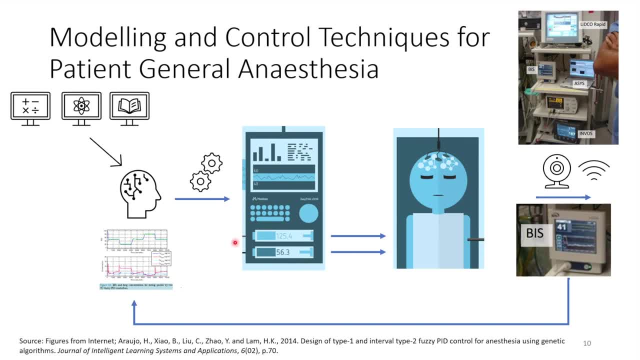 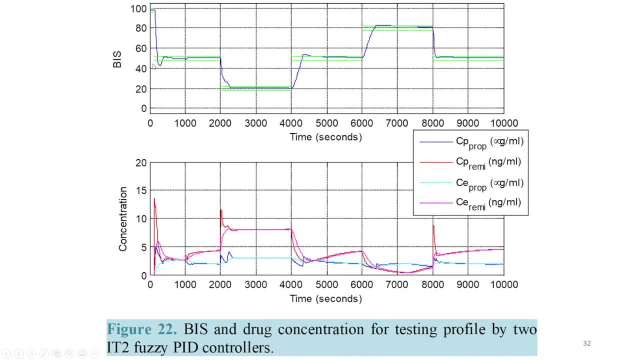 this value to around 50.. I'm going to zoom into this figure. This figure is something we have done. You can see that the green line right here, that is, we have a band of the green line. In this green line we would like to control the grids into that region. We. 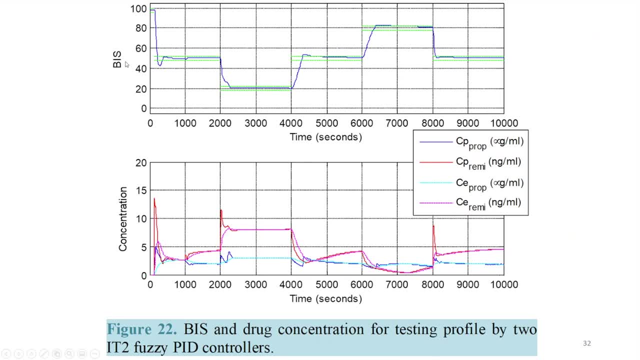 start with 100.. This is the y-axis, that is, this value, 100, it means that the patient is fully awake. We start from fully awake and then so, controlled, by injecting the drug into the patient. We are going to put the patient into sleep around 50. Going into the 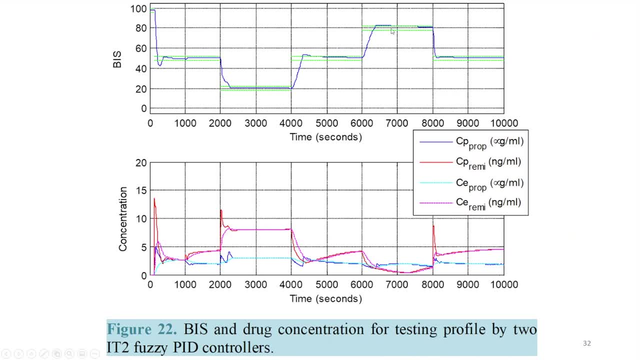 deep sleeping stages and then control it back to 50. We are doing the tracking control. That means we are going to inject the drug into the patient. We are going to inject the drug into the patient. We would like to control the green line, to follow the green line. That 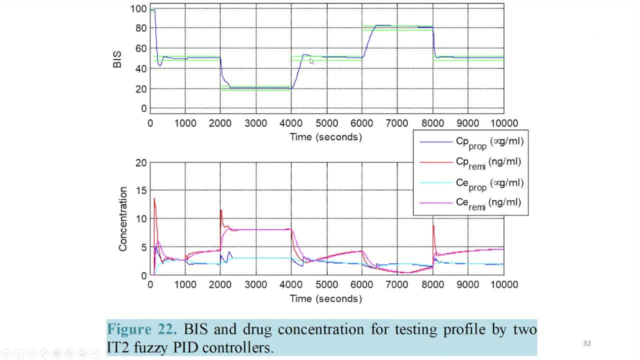 means you can see that Right here. we will give you 100% track to green line. It is because there will be some delay between the patient as well as absorption of the drug In the lower figure. that is the amount of concentration of the drug. I just mentioned the 2 jobs. 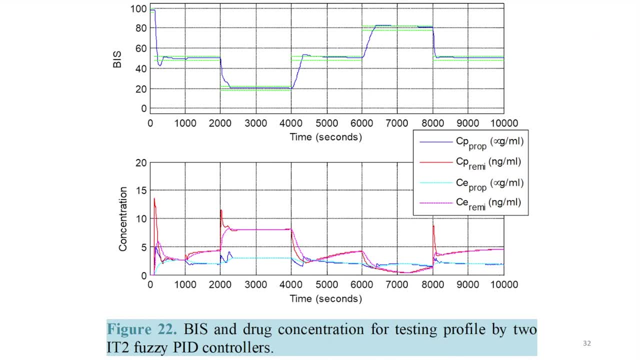 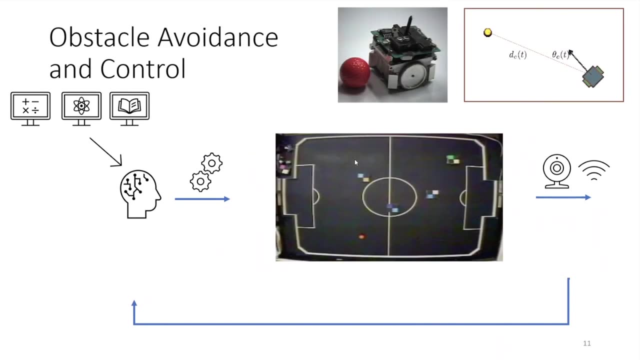 in this study. we compare that with the traditional control theory as well as the machine learning control theory, and then we demonstrate that some advantage given by machine learning power thought, and so another one that is something about obstacle, avoid and control this kind of um research. that is something very similar to the autopilot vehicle, for example. now 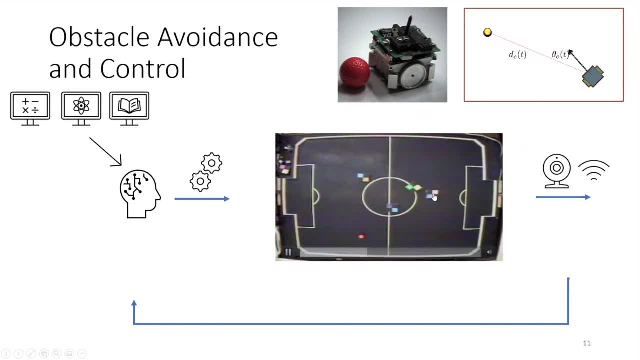 we have a vehicle right here on mobile robot in this form and that's a other free robot, and then they have a static obstacle and then we try to develop some control mechanism right here so that the robot is able to identify the obstacle as well as to pan the path. 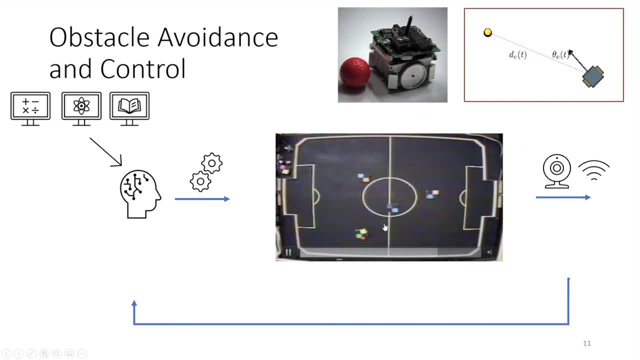 going from point a to the red one. that is the destination. yeah, so trying to do this, it is because we are having a camera on top of that, using the image positive technique to identify which robot is what it is which, according to the color code. so this is something like look at color. 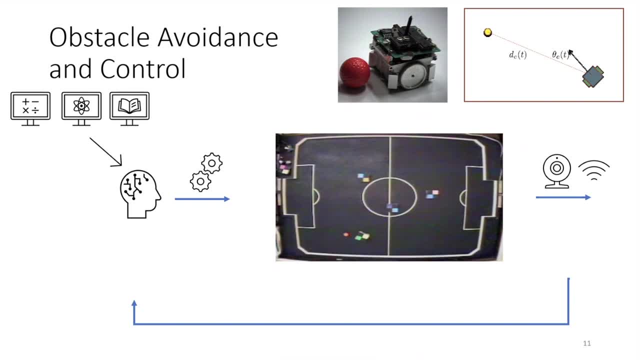 look at the robot and then look at color and then to see which robot is which, and then, based on the center of this robot, we identify the location, that is, the coordinates, as well as, based on the movement of the coordinate, we are able to finding the hacking angle, finding the velocity, so and so, that kind of information. 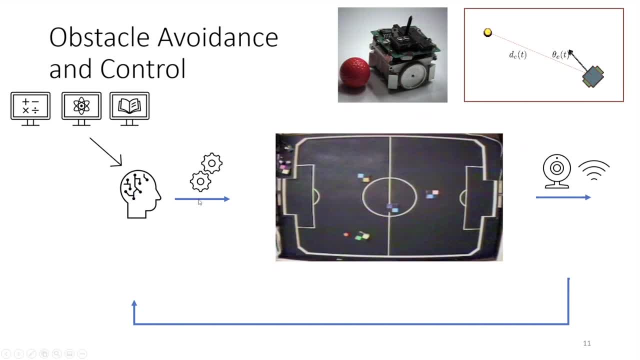 that is, will be used by the machine to make a decision, to tell which direction this robot is going to move. yeah, so that is something like we are driving and we just look at the road condition which direction we're going to move to. okay, and we have take this a step forward, that is. 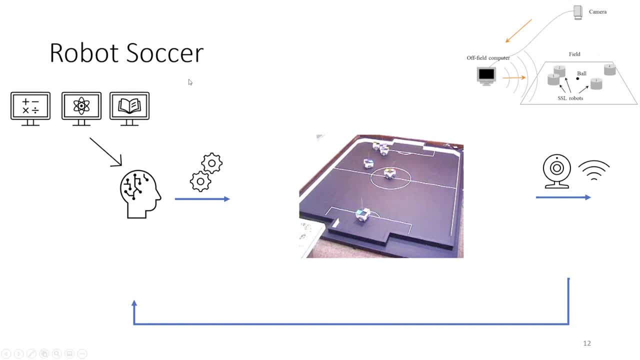 to work as a team, and then so that is a robot soccer experiment, and then so we have six robots right here. that means two teams- one side we have three robots, another side we have another three robots- and that we combine the machine intelligence as well as to control theory, to control the movement. 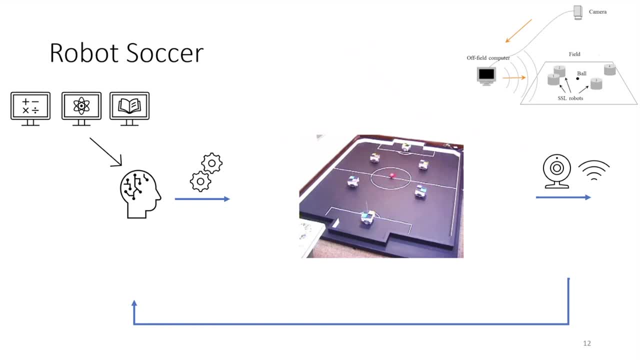 of the robot and then to make decision of the robots, so that they are playing as a team in order to get scored. yeah, so you can see that one team has better intelligence because we use, say, the grips logic and another one we just use some idea, control theory, and then so you can see the 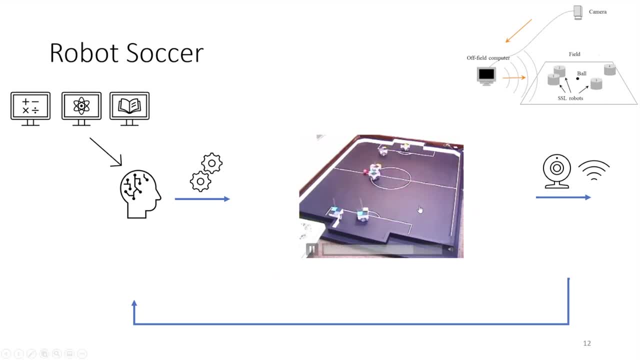 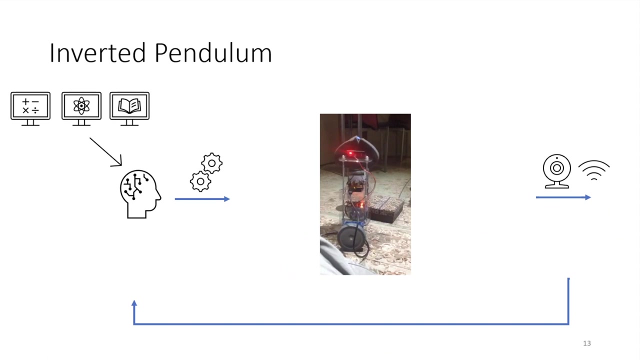 difference about that, yeah, and so this is about the robot software. still, we still use the same system with machine intelligence and learning algorithm right there. So this is the robot soccer, and we're going to talk about another simple project from an MSc student that is in pendulum balancing. 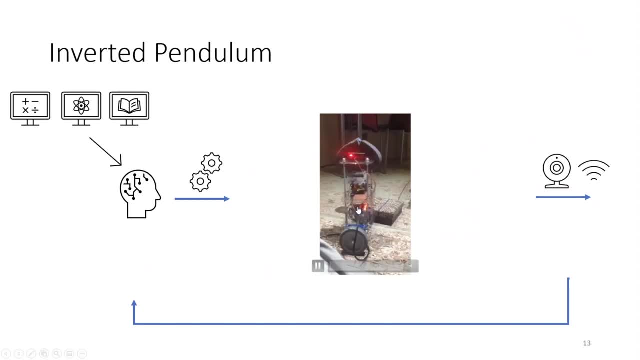 We have a robot right here and this robot it is a benchmark system and so it is something related to the biomechanics of humans, because when we are walking, actually we are an inverted pendulum. So if we are able to balance that kind of robot, that means we are able to balance. 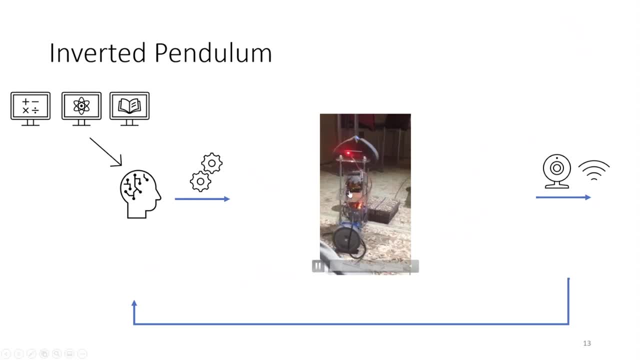 say, a bipedal robot, something like that. So we are going to measure the angle between the robot and some weapons so that we know the angle of the robot and velocity of the swing. So that's our usual robot. We are using these sensors and feed this back to the machine and then to generate the control. 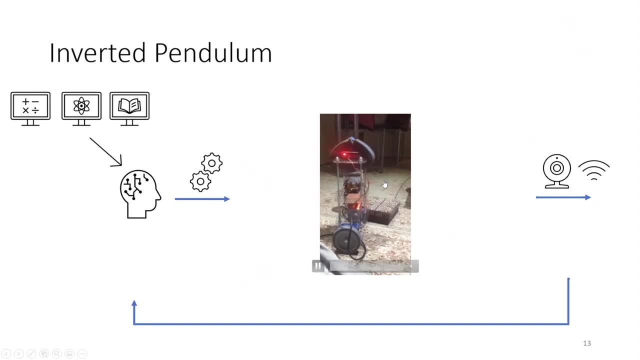 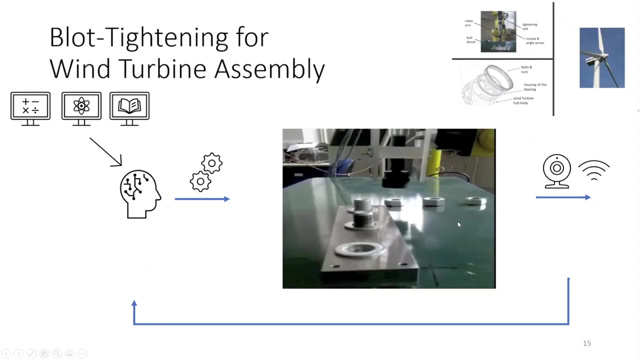 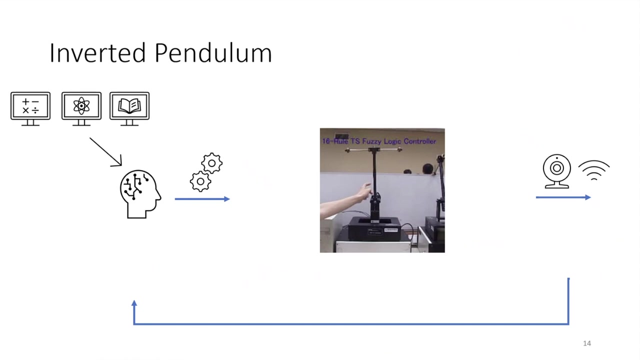 signal, that is, about the wheel, which direction and what velocity we are going to move to. The next one, that would be. So that is another type of inverted pendulum, and then so we call this a T-shaped inverted pendulum, and so the idea is more or less the same, and then so: 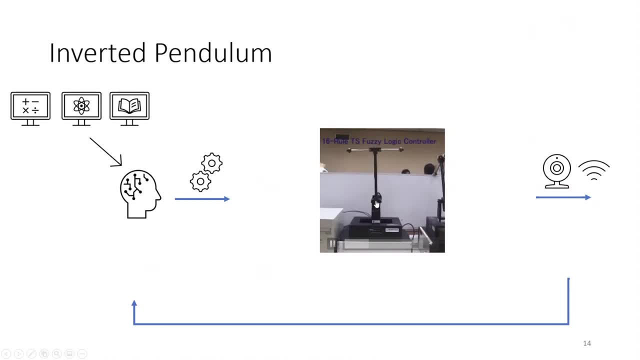 So this joint is a passive joint. It means that we do not apply any control or apply any force right here. So in order to balance the inverted pendulum, we are going to use this sliding bar. That means, right here we have a motor. 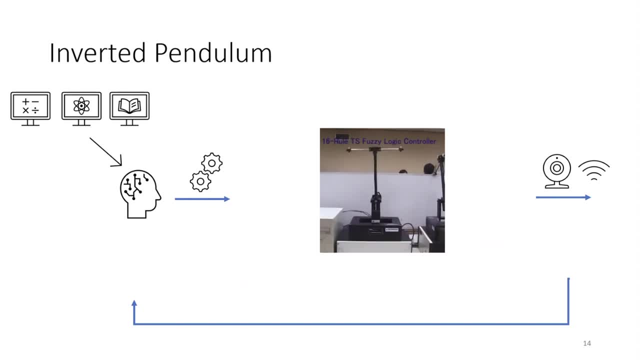 And then the motor, And then the motor will generate the signal to this sliding bar to the left, to the right, in order to balance the robot, in order to balance the inverted pendulum. So you can see that, So when someone checks the code, and then, finally, we are able to return to the origin. 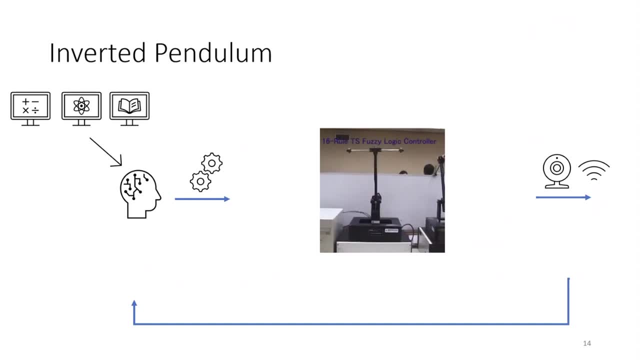 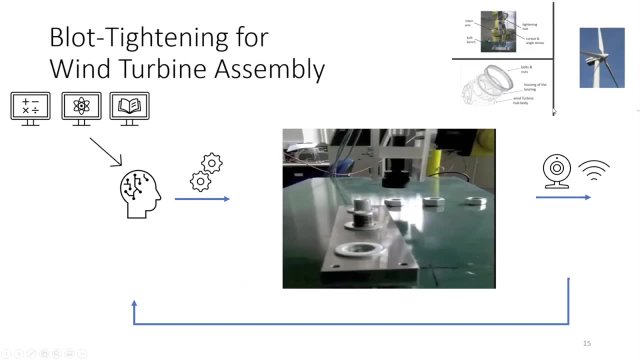 So we call this the origin. Actually, you can set the origin to a different angle. Okay, So the next one that is about an EU project. Some years ago we were talking about the wind turbine system, but in this project we focus on the bolt tightening. 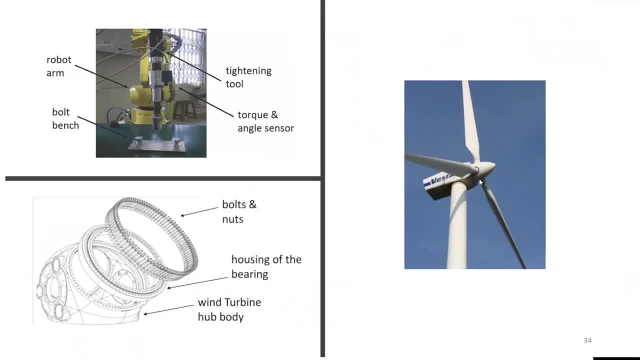 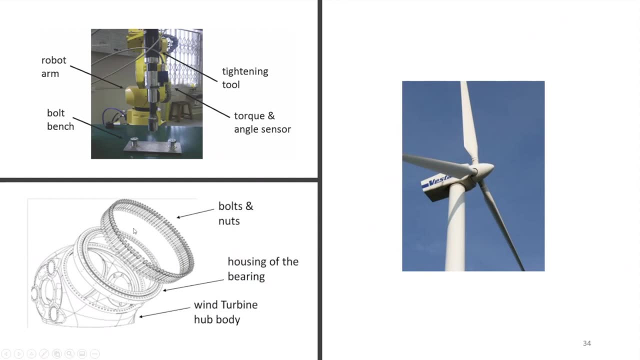 So that means when we open, when we open this up, when we open this up, we will find out that we have 128 bolts and nuts. So we would like to tighten that because in the industry we still use the human to do the tightening. 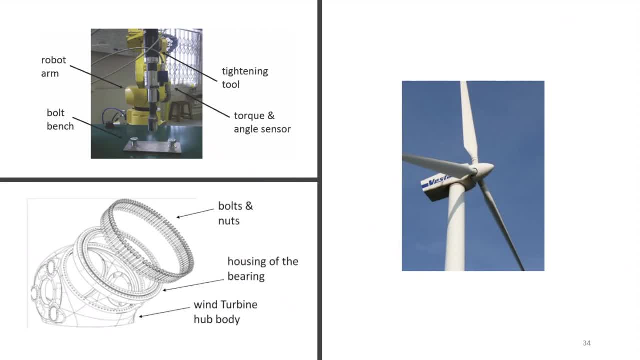 And then so we would like to make it adaptive as well as automatic. So we have done some experiments in our lab, and then so we mount the tightening tubes into this yellow robot. So we have some learning outcomes, as well as to using the buzzer logic in order to tighten. 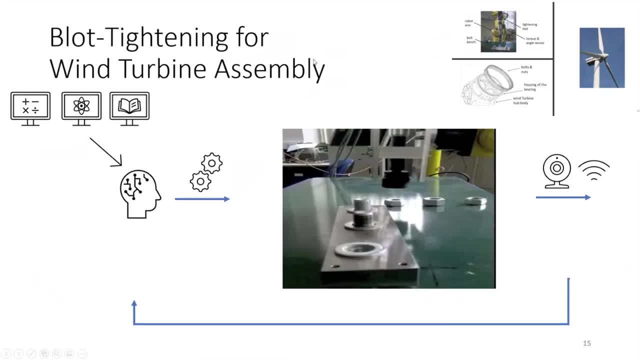 the bolt, Something like this: So this is the left side. We pick up the bolt, pick up the nut and then tighten it. We are going to control the angle as well as to talk to force so that each time, we are able to have the constant torque and constant angle. 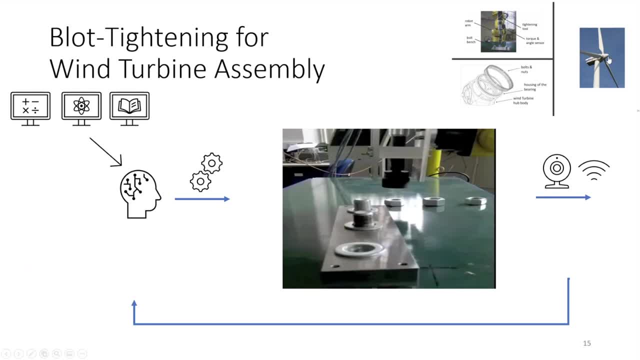 So that, so the lift this way faster in draw, So that otherwise, if the force is not there, If the force is not constant When it rotates, it will cause some damage. So we still use the coastal system right here and then. so Another experiment, that is. 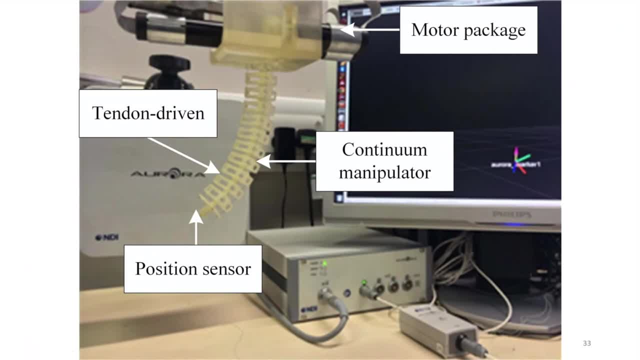 This one. we, in our lab, we use the 3D printing and then 3D print this manipulator and then so this is the tangent driven. one Tangent driven, It means that you can imagine that in my hand, In my arm. 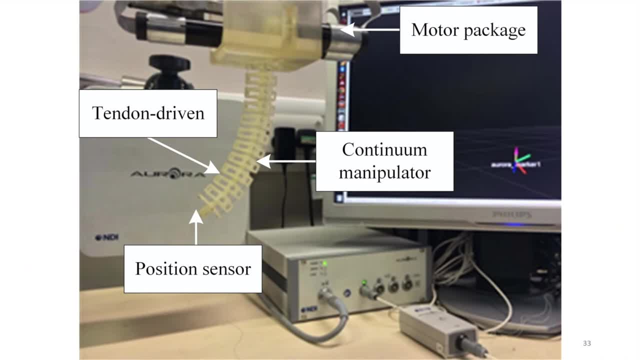 We have some muscle and then tangent, we are going to have three wires in order to just tighten it or relax it, and then we can control the end point of the arm. So we have some wires right there and then we would like to control this point. 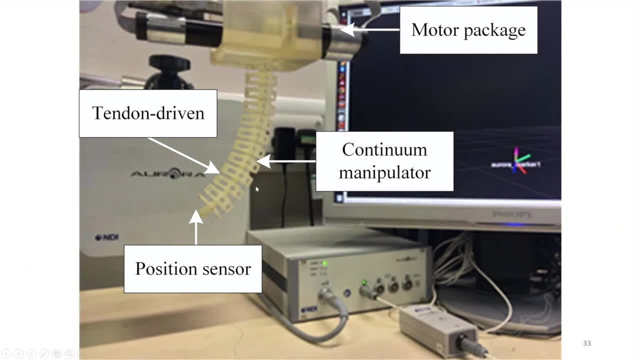 So this experiment is very challenging. It is because that it is very uncertain. We just 3D print each part of that. That means each printing it is not very accurate. and then also the tangent driven: If you are talking about model, it is highly nonlinear. and then so, if you are going to 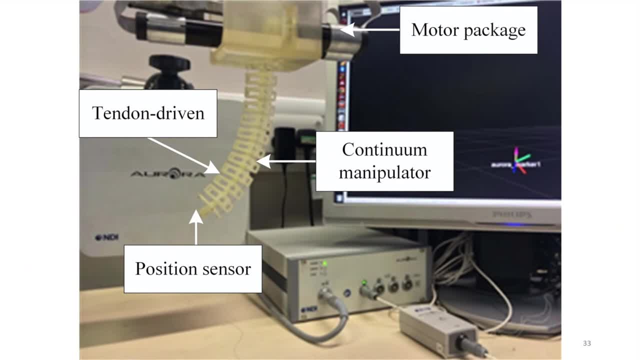 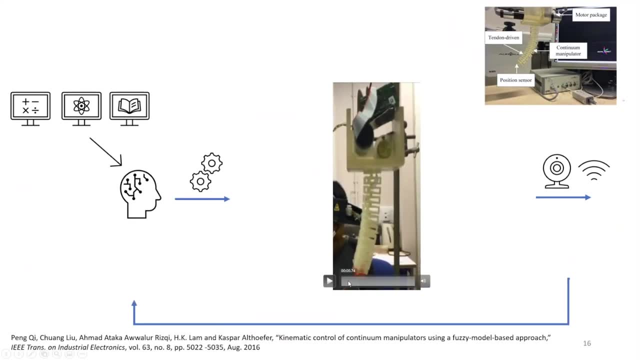 design a linear system to that. actually it works, but so it is not as good as using a nonlinear controller. So this is what we have done and then so, So you can see that the moving distance is very accurate. The distance is very short, but when we compare that with the traditional or modern solution, 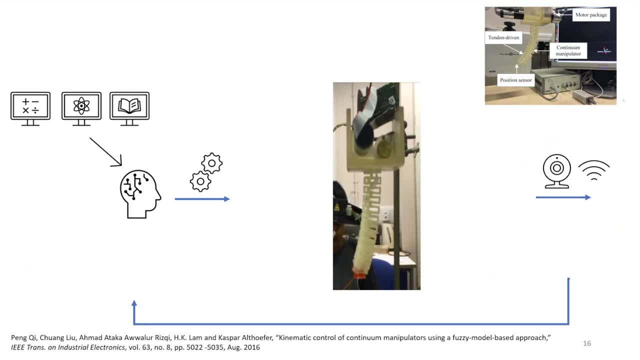 that is our method. it is still better than the existing one. Yeah, Okay And yeah because for this one there will be a lot of application, For example, in the surgery we are going to have, the endoscopic and then. so we are going to control the end factor to move the end point to certain places. 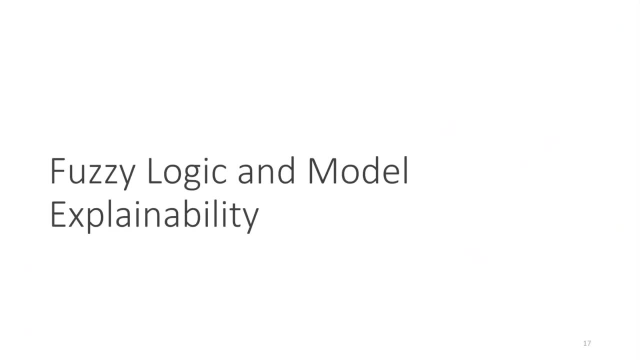 So we are going to have to do some design reporting. Yeah, So I just talk about some control theory, Some control application and then so I would like to talk a little bit more about once we have machine intelligence, then how do we interpret it? because you can just see that 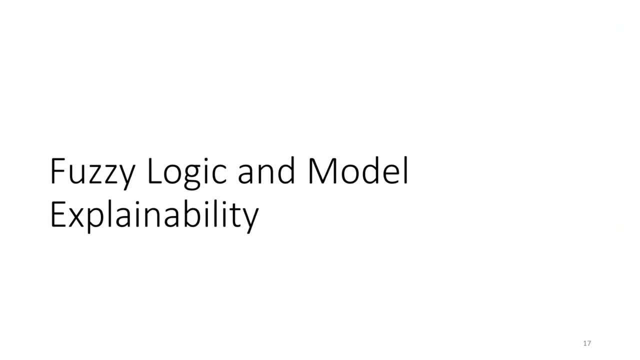 in application, it works, it works. If it doesn't work, why, And then so? So why we come up with this control policy? How can we understand something behind this control theory, Or the machine intelligence? So that is something we have touched on today. 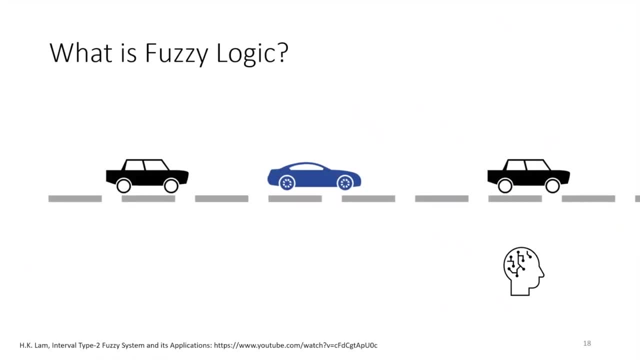 So just one slide and then. so now talking about driving, And then so we would like to drive a car and keep a safe distance. So, for example, this is the blue car is driving, and then so I would like to keep a safe distance. 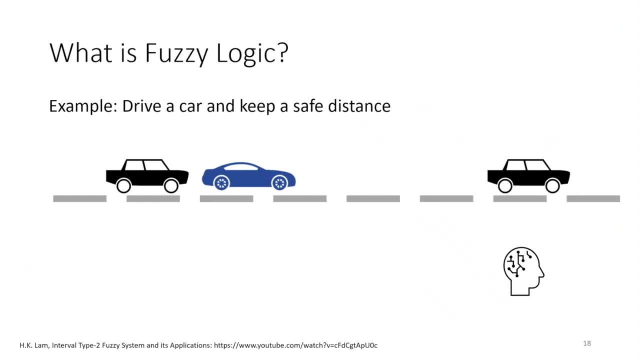 But the thing is that what is the safe distance? We don't know. So that means different countries, different places will have different rules. So that means it is something very weird. But the thing is that if someone told me that I'm going to drive in a safe distance, 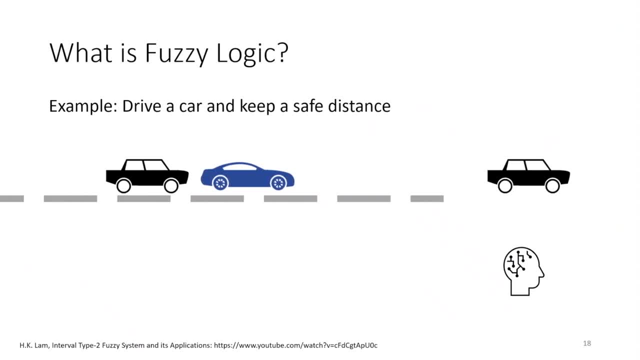 in my mind I come up with some rules, So these rules, that is something like that. So if the distance is small, for example, this distance is small and then. so I'm going to keep the speed to be low, or I do not accelerate that, or I'm going to decelerate. 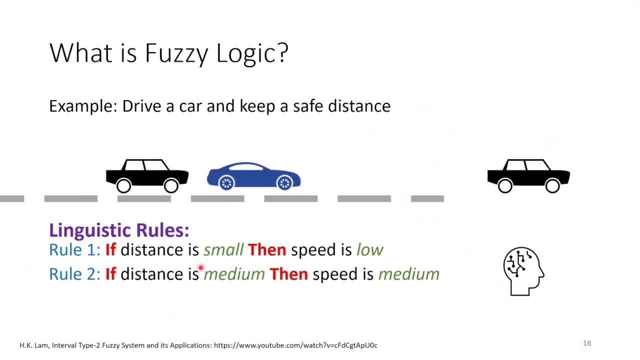 And then what about if the distance is medium, For example, in this position, and then I should control the speed to be medium speed, and then so that's what that would be. That's it. Distance is large, Like this case, I'm going to increase the speed. 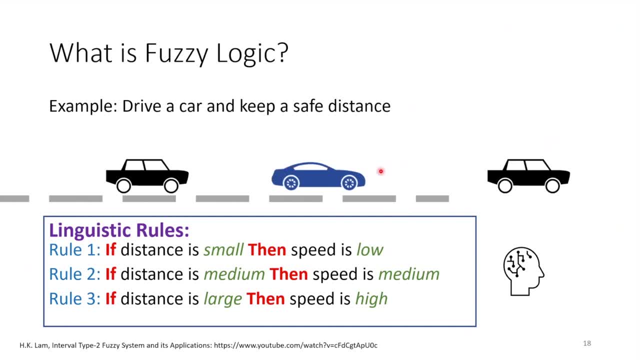 The speed is high. So that is something in our mind, But the same thing is, how do we understand that Linguistically? we understand what it means, but what does it mean by small? Because when we talk about small, whether this room is small or we're talking about, 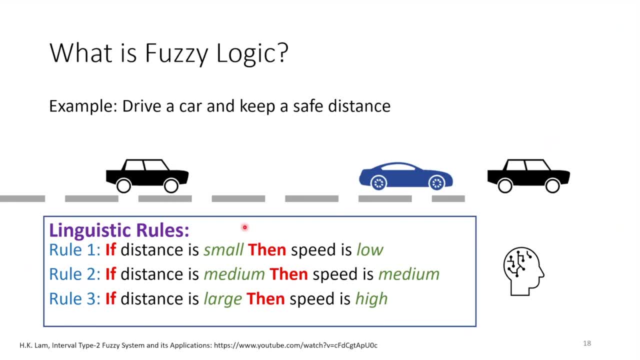 the distance is small. we use small to describe a lot of things. So anyway, later on we have defined what's small, what's low. Actually, this language to turn we have defined, But in general picture we understand what it means. 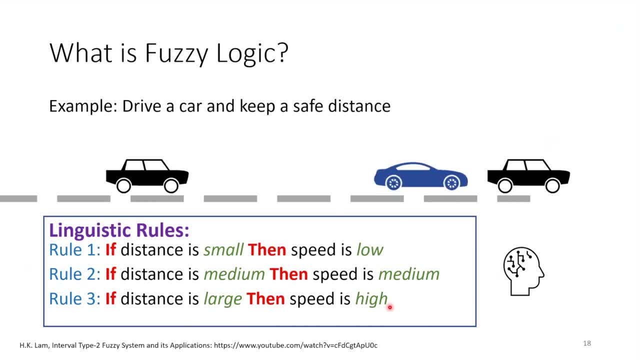 These three rules come out together, which give us some ideas how to drive a car and keep it safe from distance. So in this case, if we're able to have a machine learning, our software automatically develop these rules and then we can explain to the machine intelligence. 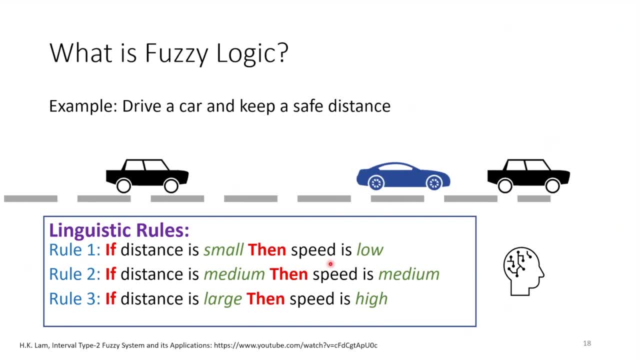 So we know what the machine is doing. So this is one thing. Another thing, that is, if human, we can provide this rule to the machine, that means we're able to teach machine what to do. For example, this morning we talked about 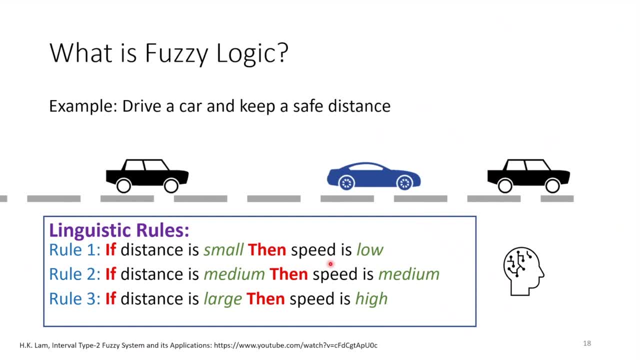 to determine whether the chemical is toxic or not. If we're able to come up with some rules and then if this chemical or this complete всех or this company has this kind of features, and then most likely the final product will be toxic or the risk level is maybe low, high or something. 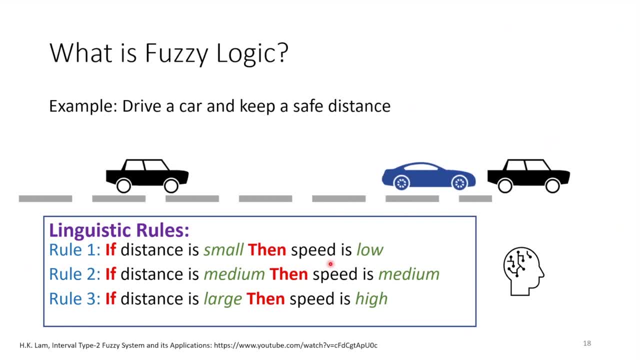 So in that case, that means at least we could be able to incorporate our knowledge into the machine intelligence and then so, In return, this machine intelligence can be explained to us. We can understand what the machine is doing. so that's why we can use the methodology to do this. 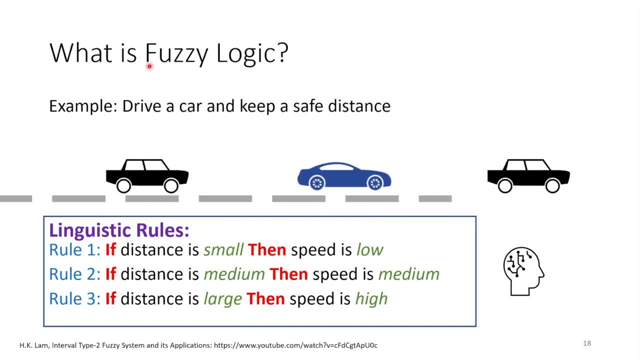 So that means in this case, this is the model-based explanation, and then so there would be something like model-free explanation. we call that model agnostic approach. So that means when we have deep learning, it is an object model, a encant box. 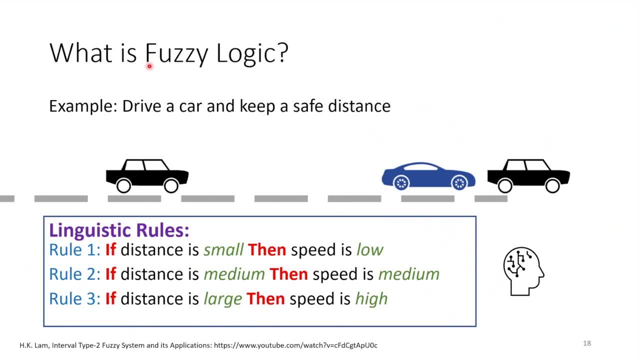 We cannot explain that, but we have some algorithm Or some mechanism to explain it. For example, using the mind, using the software, we can have a snapshot of the input to explain why the output, why the machine made that kind of decision. 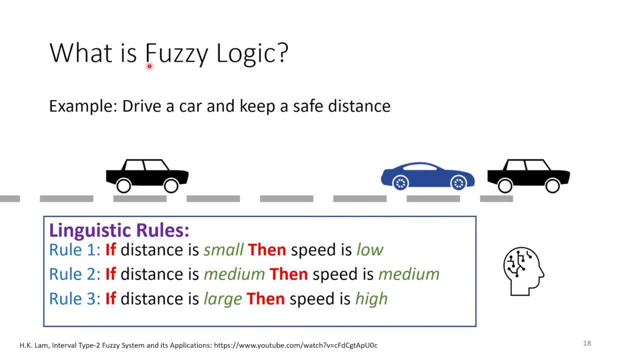 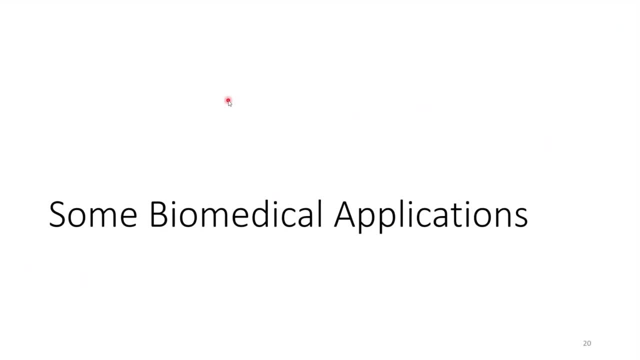 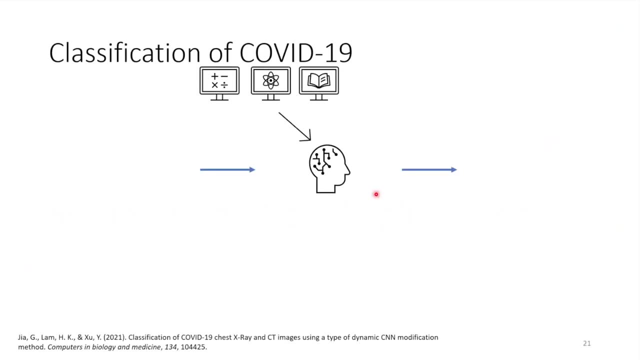 But anyway, the first logic, that is, we are able to develop some groups. these groups, that is human, can understand. So I'm going to talk about some biomedical applications. So, classification of the COVID-19,. our team has done something about that in the past. 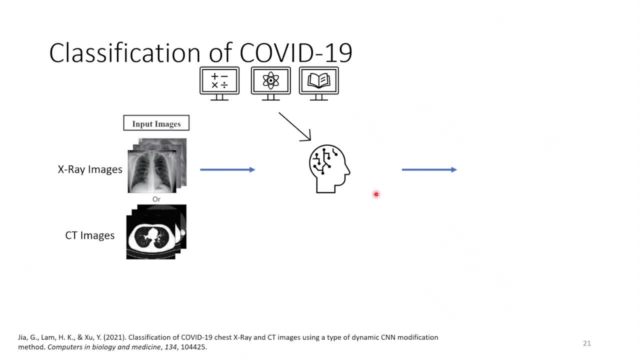 two years. Now you can see that I'm going to turn the closed-loop system into an open-loop system. This open-loop system, that is, we have input and then feed it back into the machine and then the machine is going to generate the output, and so the input in order to classify. 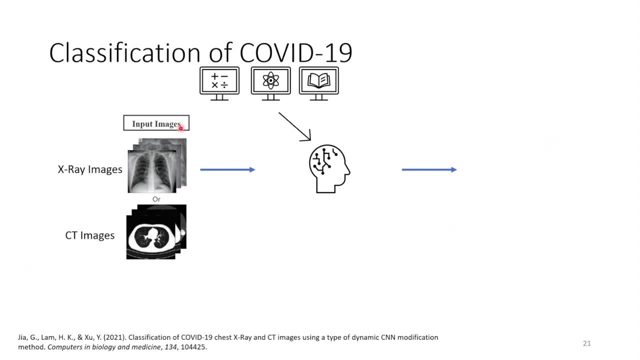 whether it's COVID-19 or not, We use input images, for example x-ray image or the CT scan or something like that. So in this paper, and we use these two kinds of images. So model, right here we use a bunch of model, for example some existing models. 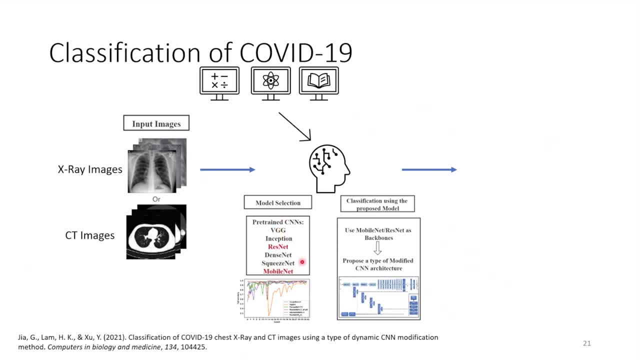 I'm not going to read that out, and that's for example. all of them are CNN model, convolution of new network learning model. We make some modification and so this model is able to classify five, five classes, for example COVID, pneumonia, normal or tuberculosis, something like that. 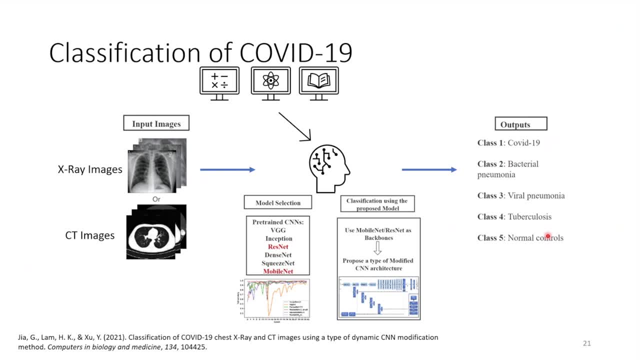 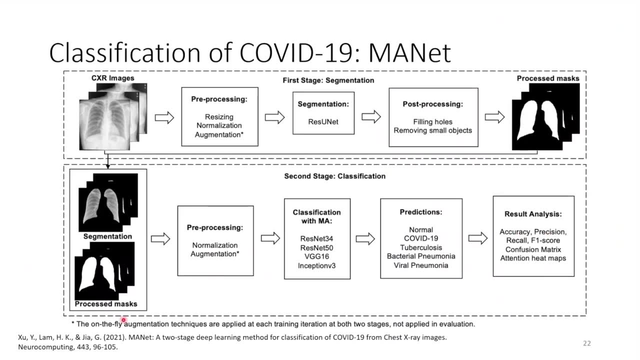 So that means if you're going to increase the number of classes and then you retrain the model and then it's effectively done, The next one and the paper doing the same thing. that is about classification of COVID. So we use the new model. 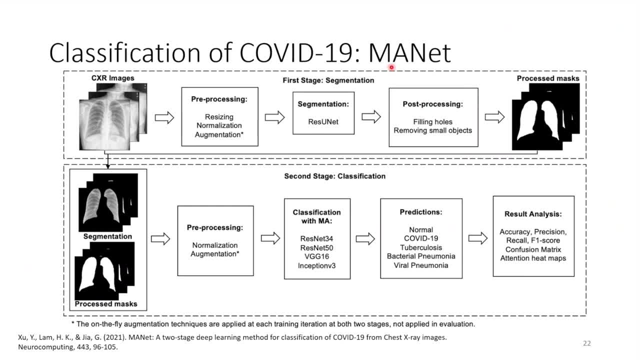 We use the new model. We use the new model, We call this the MA lab. The MA lab, that is, we use the attention mechanism, Attention mechanism and just some kind of at least in the machine learning. So the idea is that because in the previous slide, when we do the classification, we just 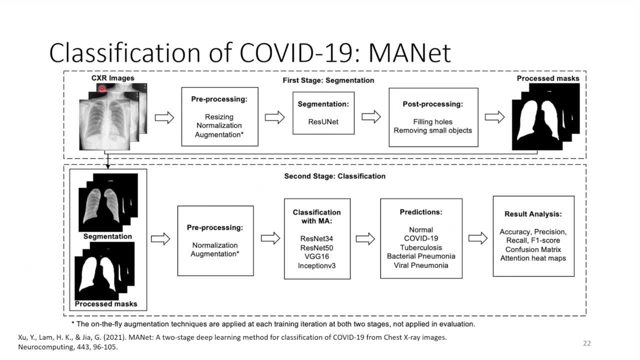 take the whole image, just like if you say I need the whole image and then so, based on this whole image, I'm going to determine whether this is COVID or not. But the thing is that if we think about what the human is doing when we look at the X-ray, 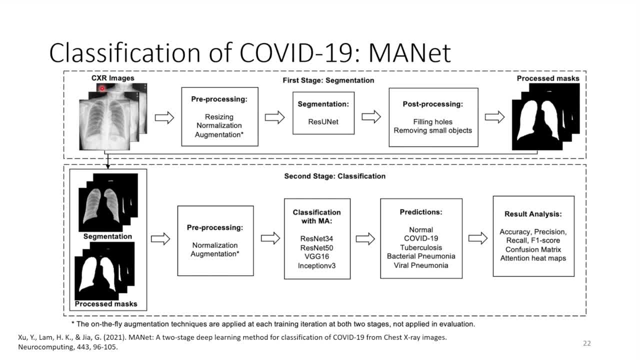 image. actually, we're going to focus some features. These features, for example, because the COVID, the features coming from the lung section. So we're going to have some mechanism, the attention mechanism that is to figure that out. amongst that is the lung and then so 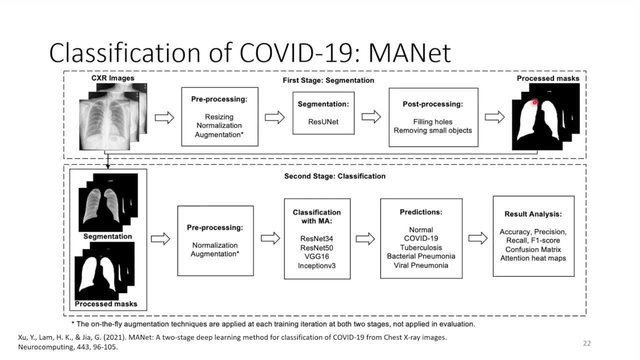 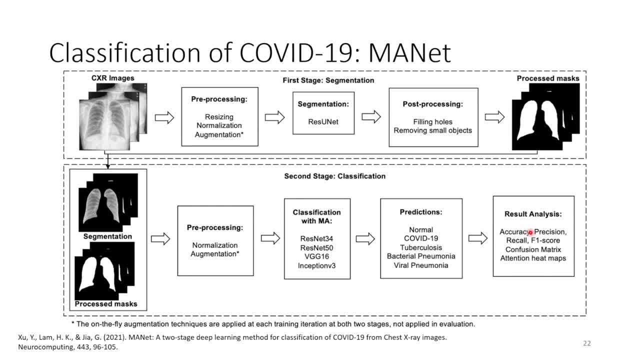 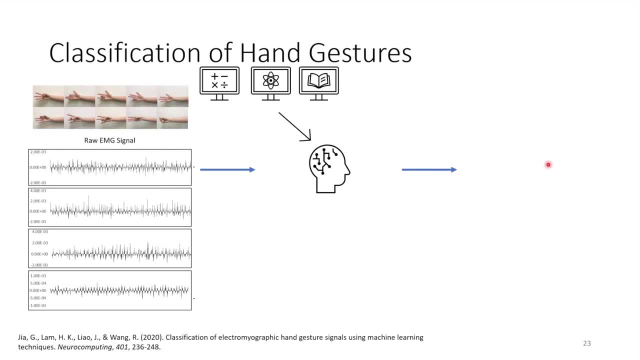 it is COVID or not, or other causes And some other classification application. So this one, that is, we capture the ENG signal. The ENG signal That is some signal from the lung, That is some signal from the muscle. We are going to say we would like to control post-practice. 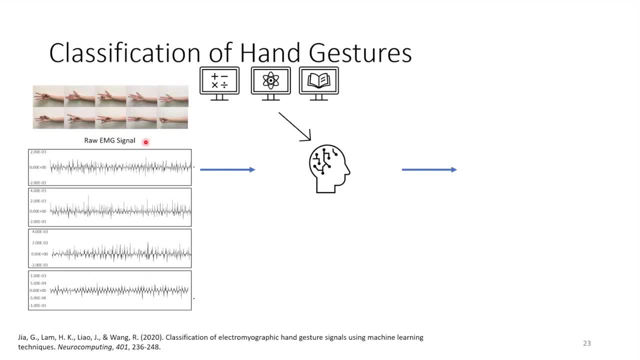 And then so moving this muscle using some sensors right here, And then so this muscle, the contraction of the muscle, will give you a different kind of signal. This kind of signal, we fit it into the CNN model or whatever model, And then so we can tell you that what kind of gesture this person is going to make, or 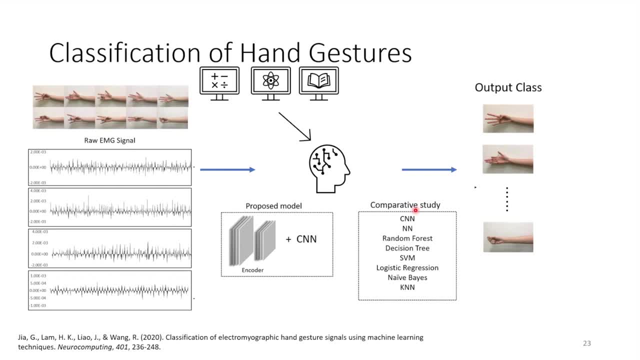 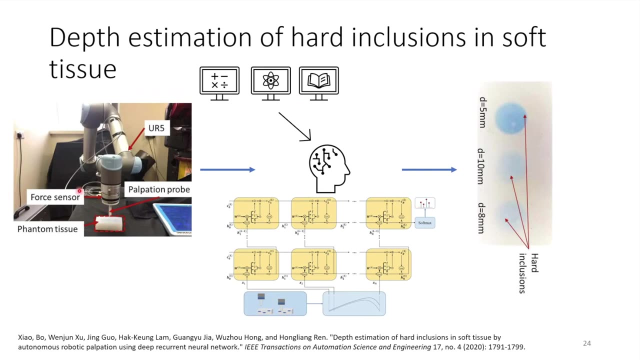 doing And then so so that we are able to control the post-practice or whatever machine. yeah, Because if you're doing the remote control and then so we can still use this kind of technique to do that. So another one. 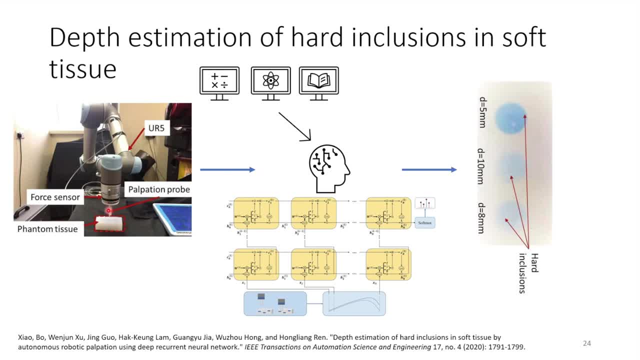 We have a global When we look at this one, this is the, this is the full, a propulsion probe that is something like a finger And then so, in the surgery, We would like to, We would like to. In the surgery, we would like to determine whether there would be some heart condition. 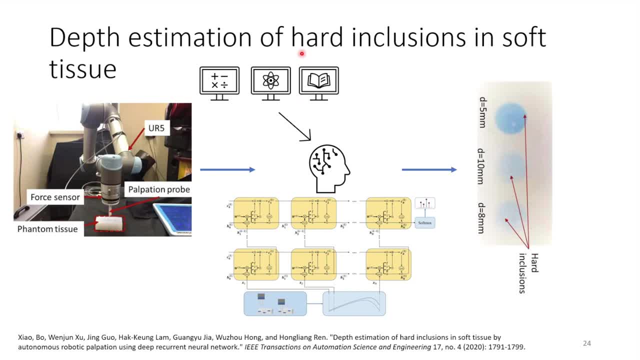 say tumor, And then we're going to slide our finger. the surgeon is going to slide finger into soft tissue And then to feel whether there would be something down below, And then so. so this is something using robot to do the human job. 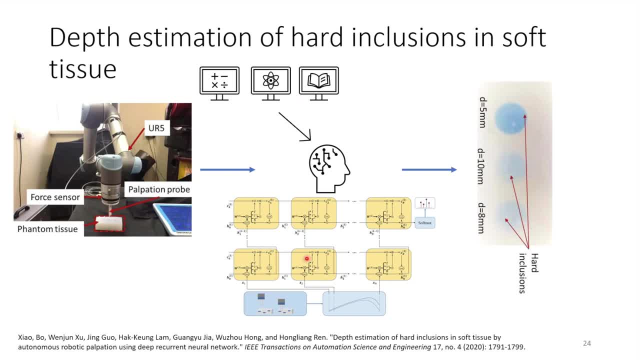 And then so so we use the LSTM of the long short term memory, And then so this is A kind of machine learning technique, So this is the finger slide along the tissue, and then so we collect some signal, fit this signal into the LSTM to capture the spatial as well as temporal information. 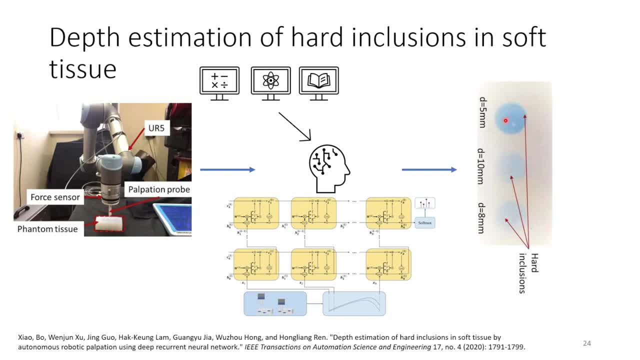 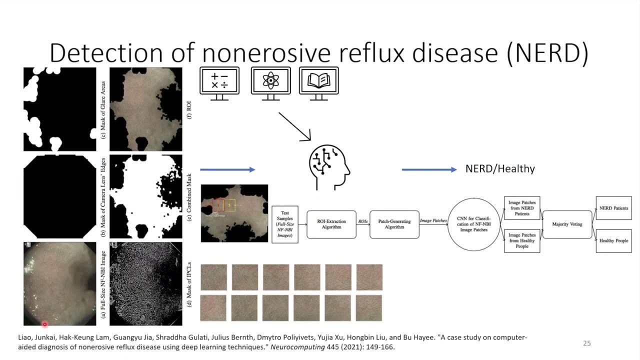 And to determine the depth or the size of this heart inclusion, that is, the tumor, for example. And so this is the paper, And another one that would be Okay, Okay, Okay, The data set from the King's Medical School as well. detection of long erosive reflux. 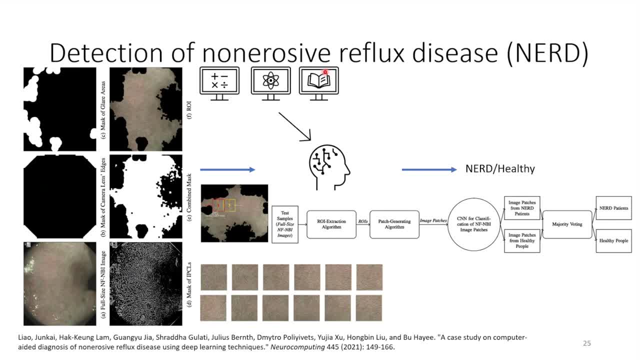 disease. So that is something like we have some stomach acid which is reflux to our esophagus So that it caused some damage right here, And so what we're going to do is that to insert the camera and then so to look at, to look. 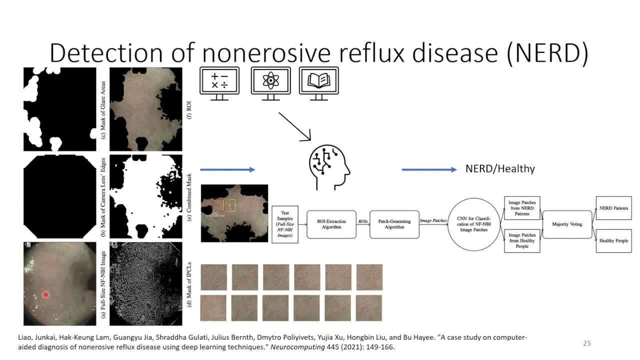 inside, You could find out that there's some image right here, And, in order to capture better the features, we're using some techniques to mask out some non relevant information, And so, throughout this process, we identify this region And then so we are going to create some small patches. 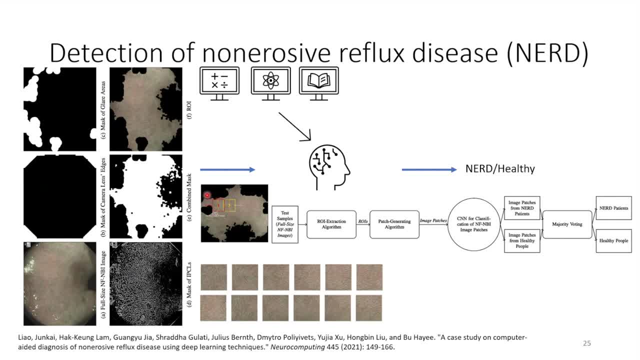 That way we are going to look at region by region, one by one, And so if you're going to slide a window From the left To the right, So if you write from the top to the bottom, you are able to come up with these small image patches and then so fill it into the model, and then the model will just tell you that this small patch, whether it is burnt or not, so that is healthy or unhealthy. 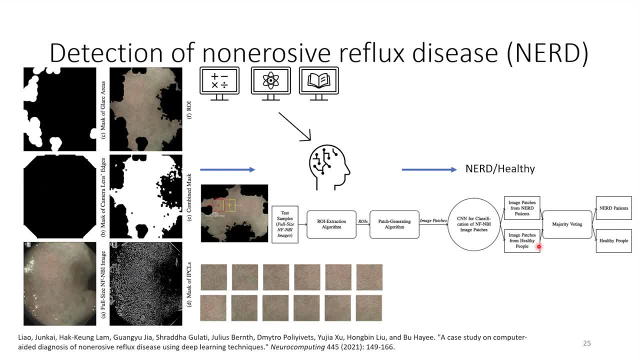 So after a sequence of these small patches, we can, after majority, rotate. That means this is positive, this is negative. If more positive than negative, then we can tell that this is positive, Otherwise it is negative. So something like rotating. 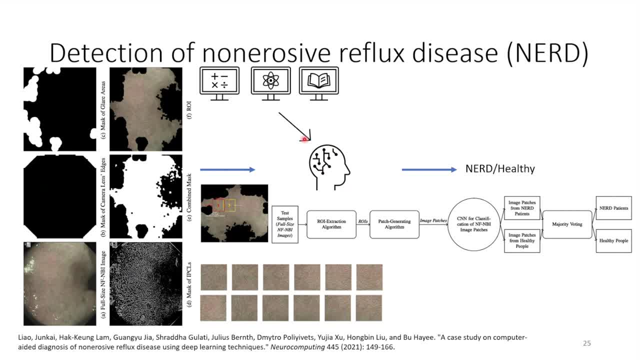 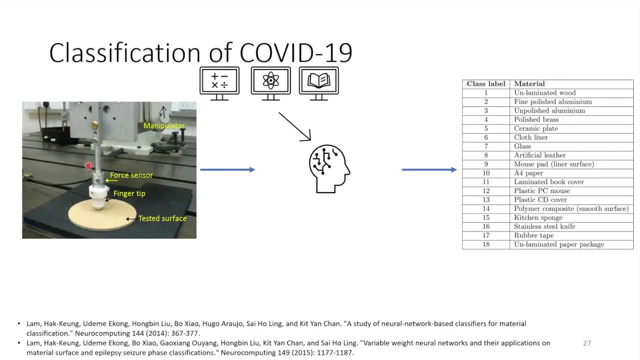 So this is the application using the machine learning. So we have some learning how to tell what parameters we are going to use in the CNM And the next one, some in this real applications as well. So this one is something very similar to to have impulsion detection. 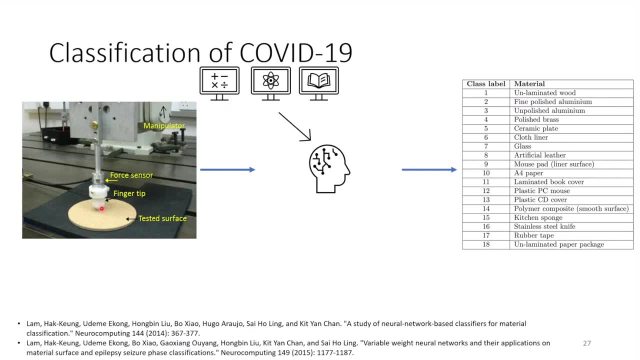 In the lab we have the tactile sensor. The tactile sensor, that is, we have a finger which runs along the surface and then to feel the texture of this surface, and so this one will just tell you that what kind of material it is. 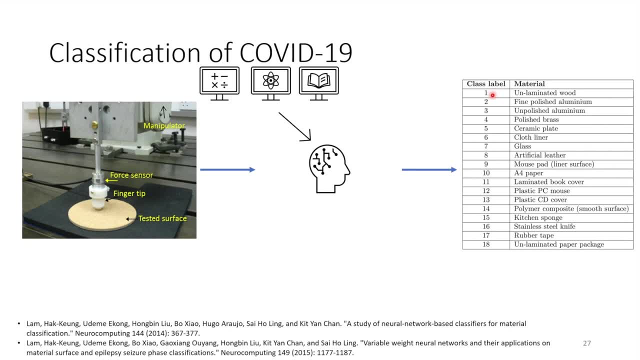 For example, if we would like to have a robot, the robot is going to grab something, because when we grab something it is a hard, hard root, And then so we are going to use some, say, ball force to grab it. If we are going to grab an egg, and then so of course we cannot just squeeze on that. 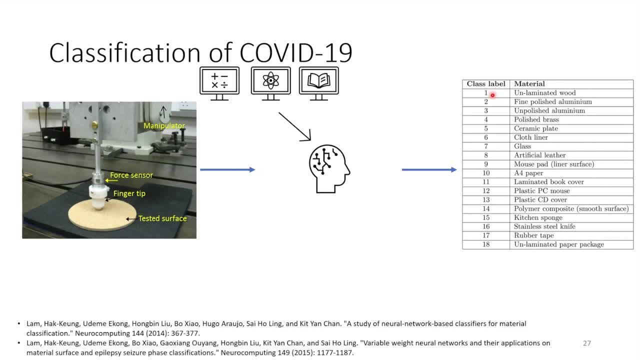 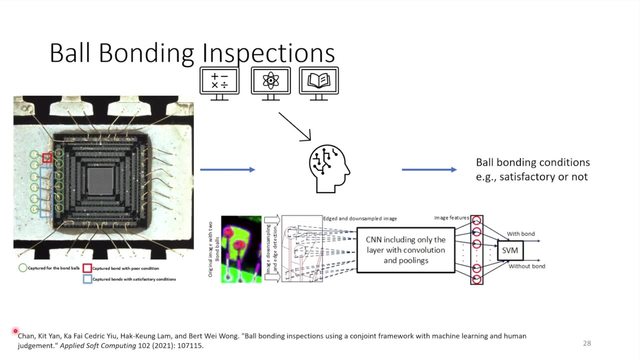 So that means, by identifying the texture, we are able to control the force of the robot arm and then so to control the friction So that we are able to practice it. So these are two papers, And so the next one, this is about the ball bonding inspection. 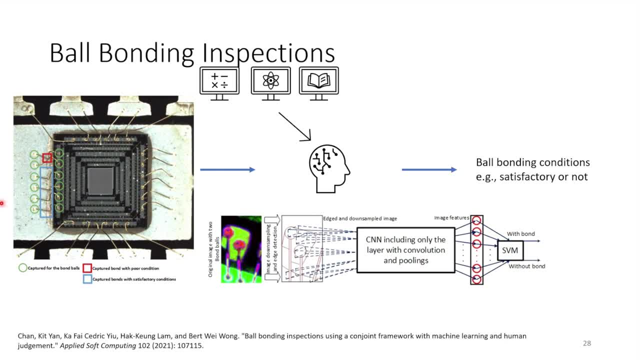 So, to explain this better, that means when we are going to open our computer, our laptop, then you will find something right there. That means we have an integrated circuit. we are going to use the solder To solder to solder all these integrated circuits into the circuit board and then so. but if the soldering is- I mean the soldering condition- is good or bad, it will determine whether this computer works fine or not. 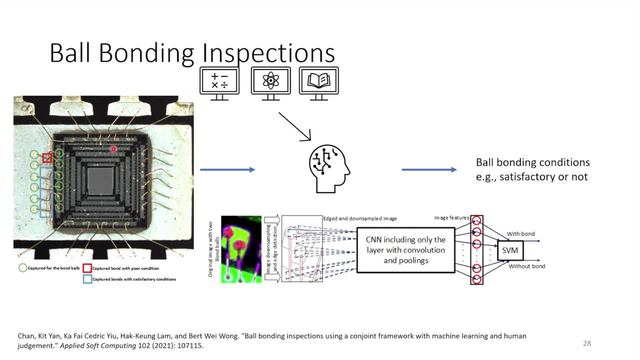 So we are going to have an algorithm using the image, take a picture, or we are going to have a camera slide along this circuit board And then identify the bond location and then check whether this bonding condition is good or not. And so we have some mechanism or machine learning model in between fitted into the machine and then just to tell you that the condition of the bonding. this is one application, and so this is the paper as well. 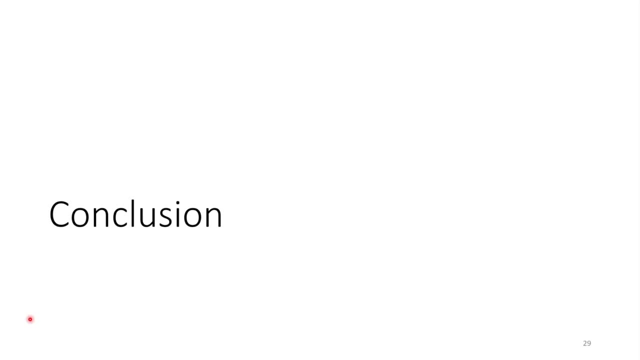 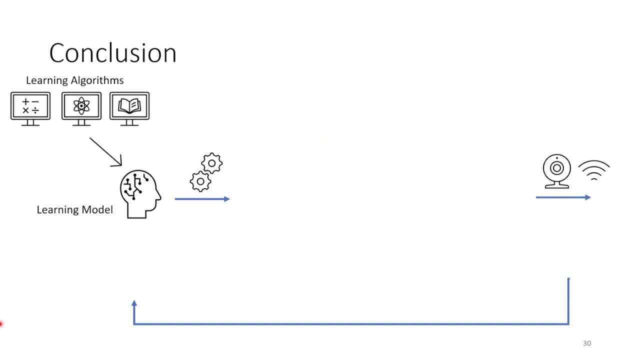 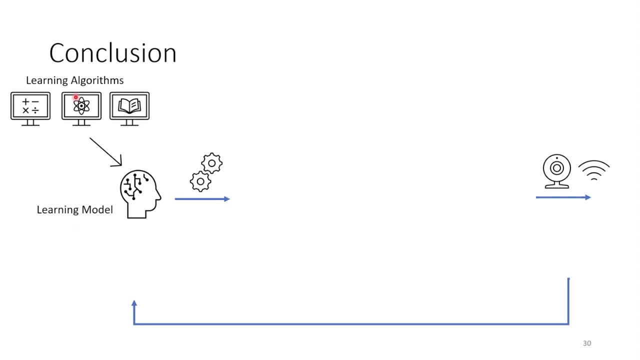 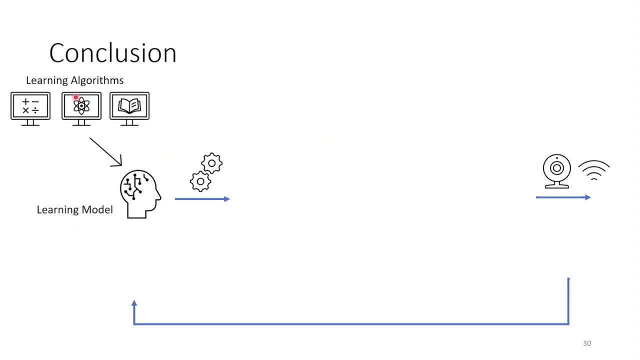 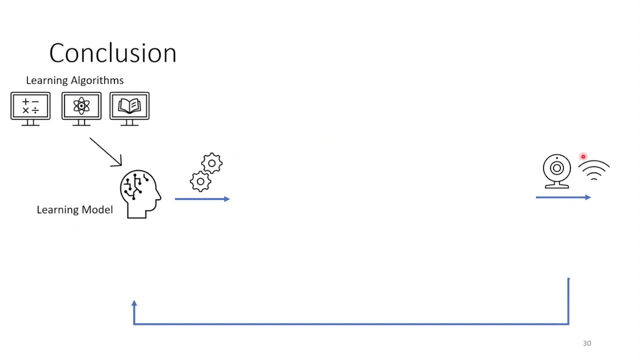 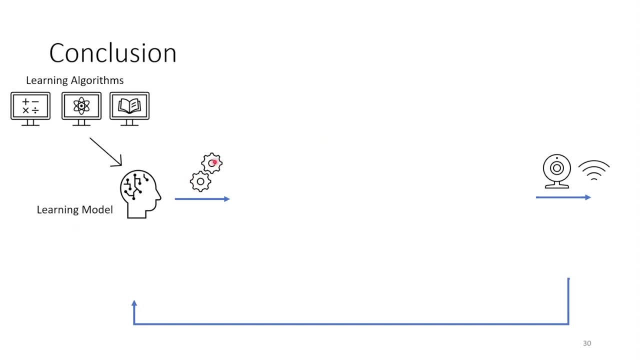 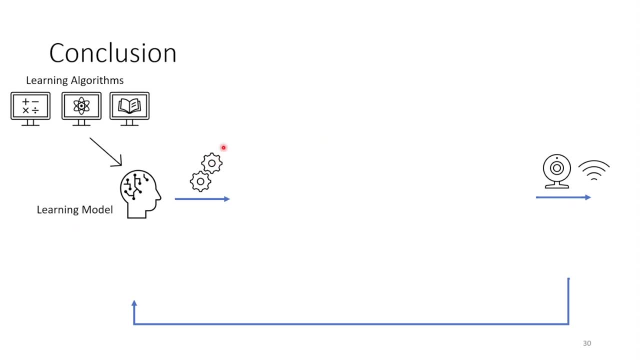 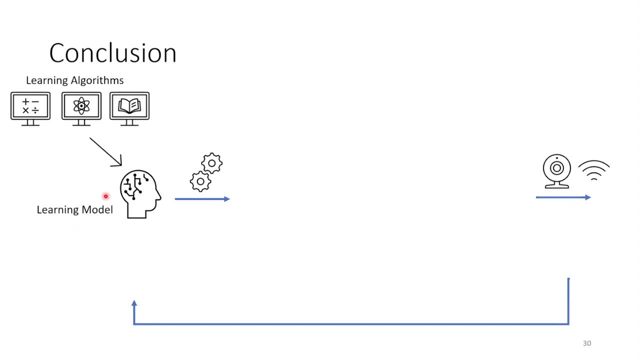 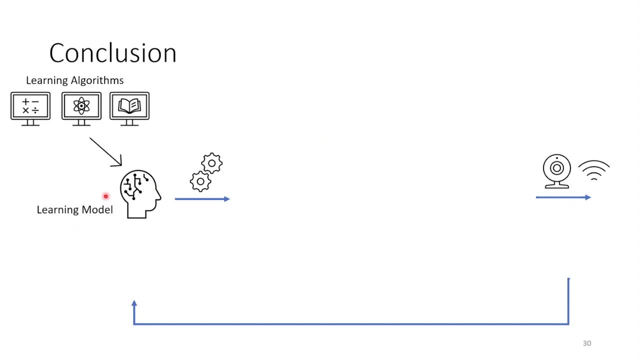 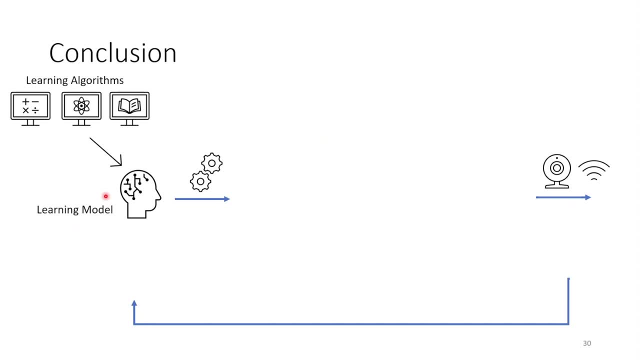 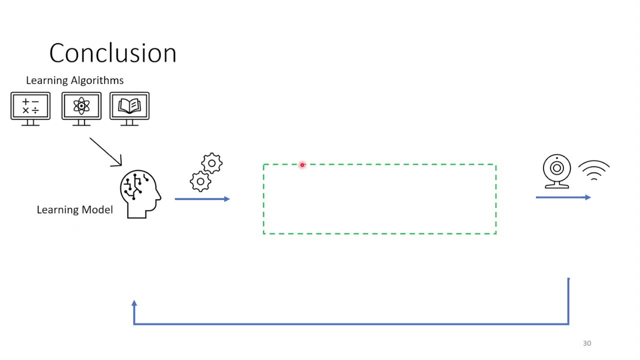 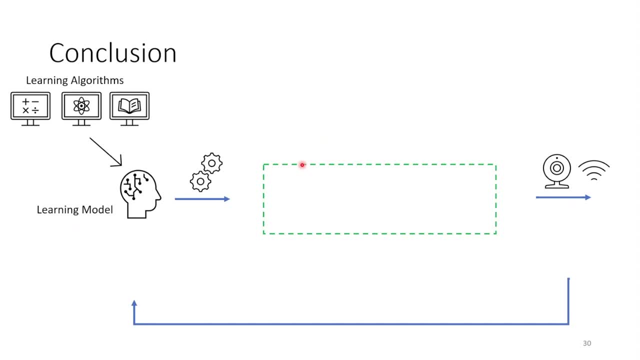 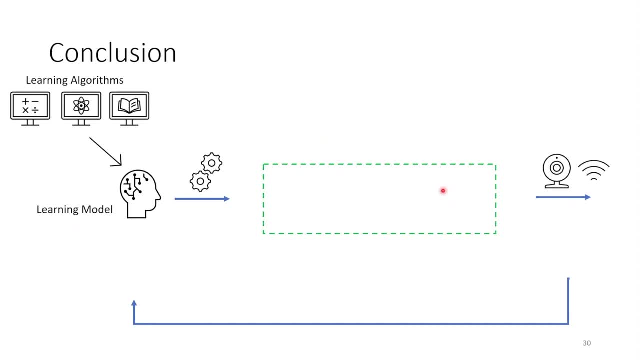 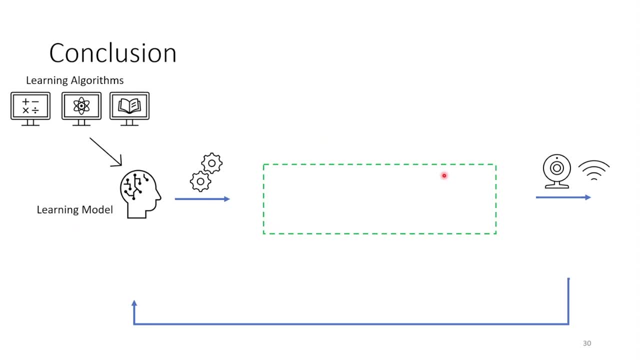 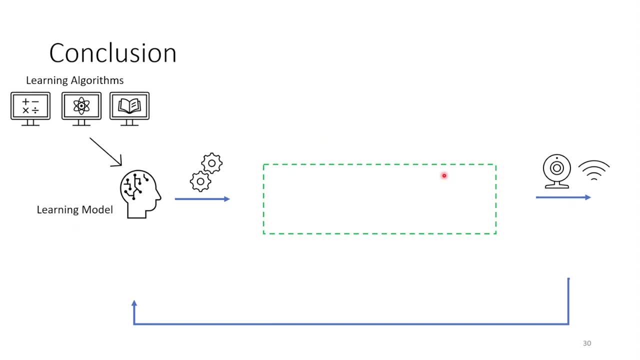 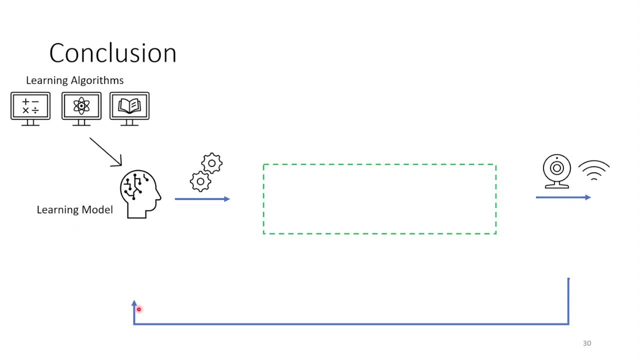 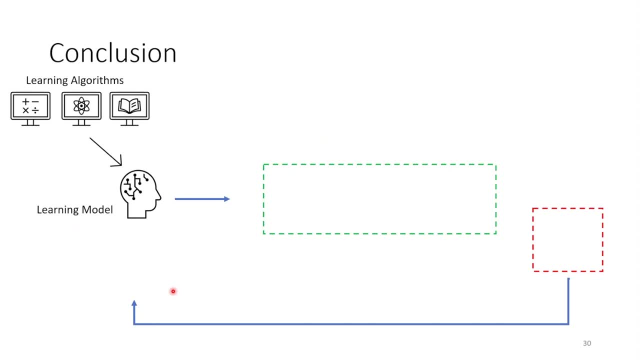 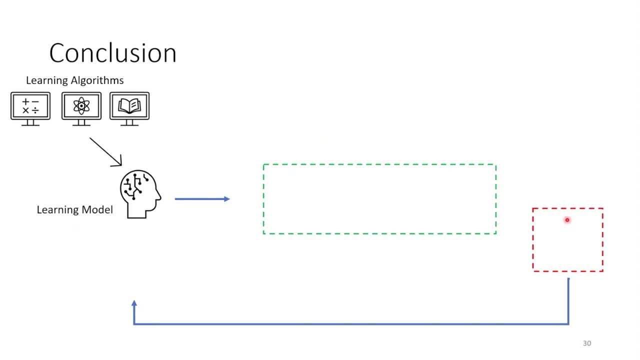 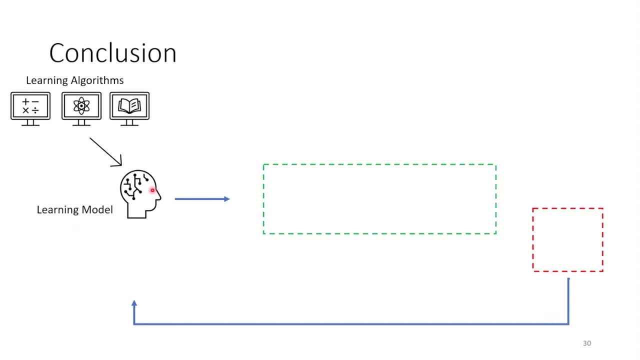 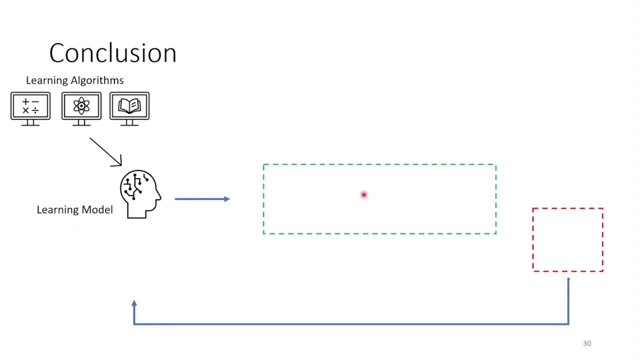 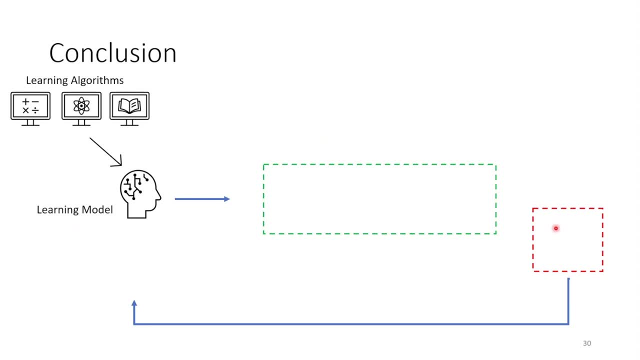 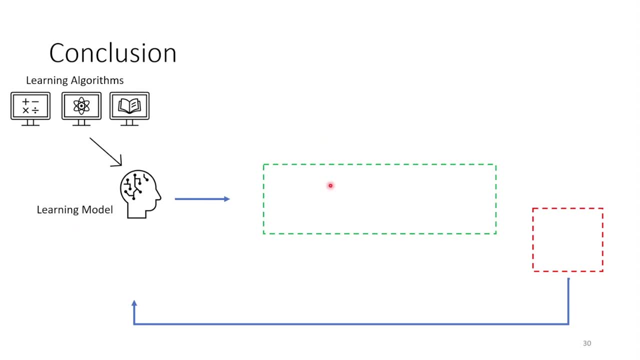 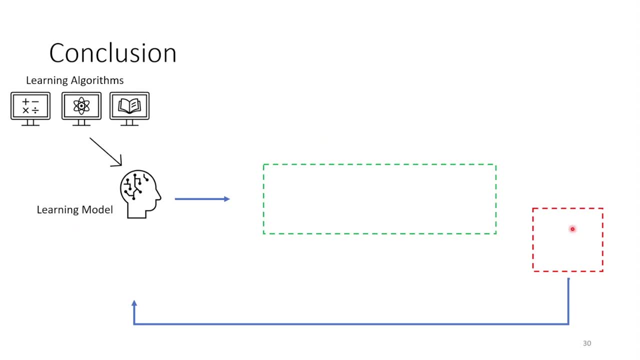 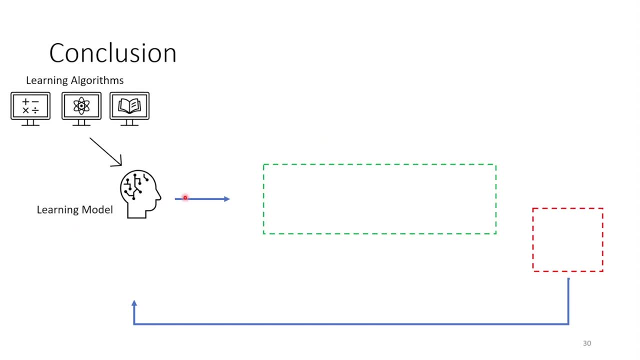 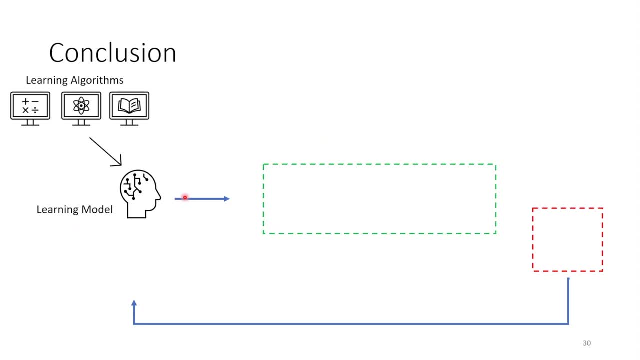 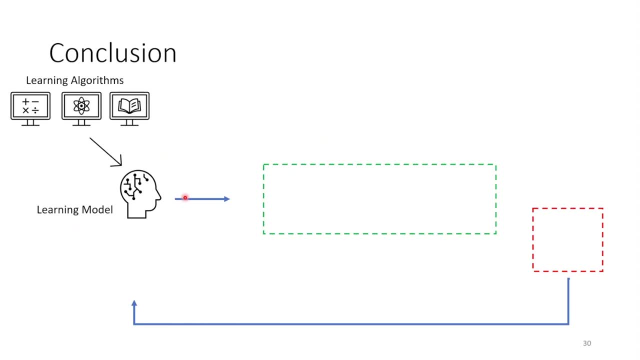 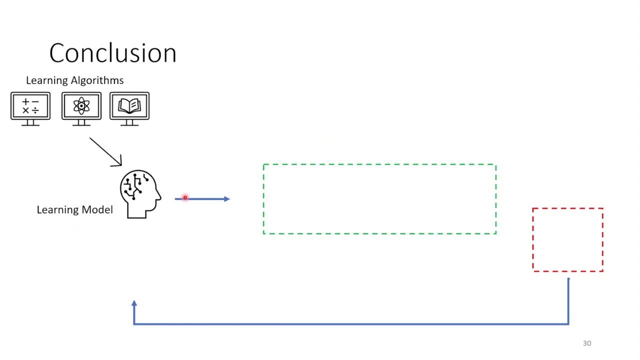 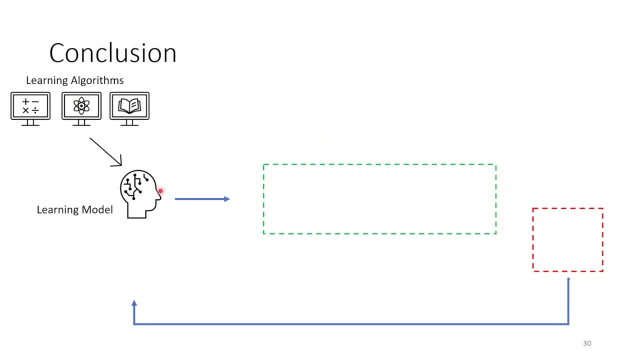 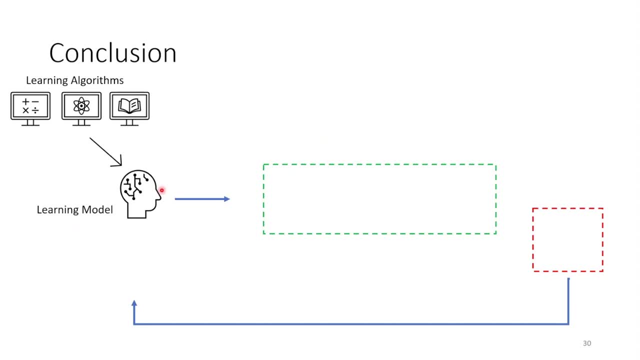 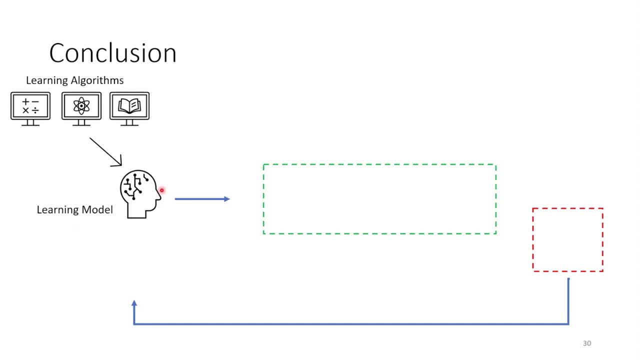 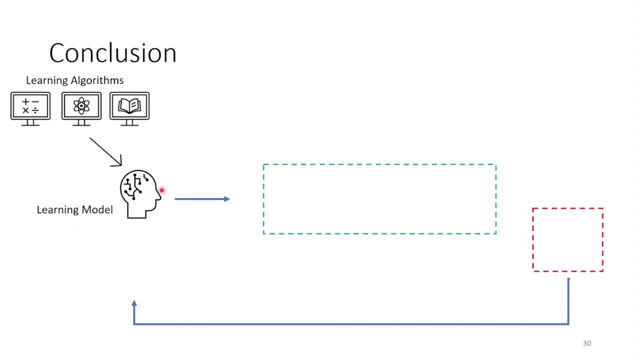 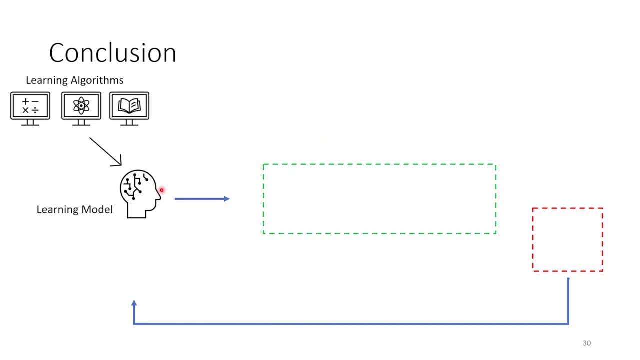